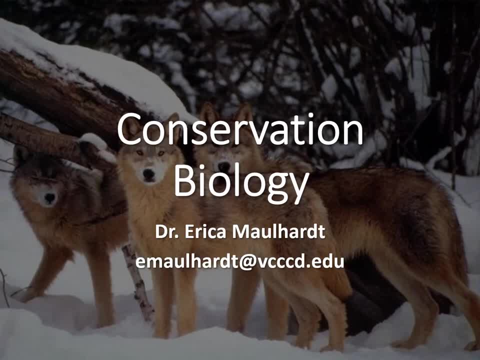 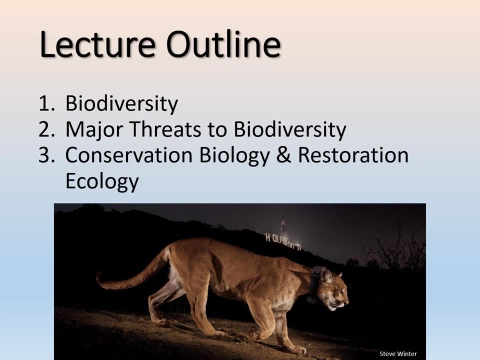 All right, you guys, welcome to our final lecture, and the last lecture for this unit. We will be discussing conservation, biology as well as biodiversity. So first we're going to cover biodiversity and kind of the changes in biodiversity that we've seen historically, as well as kind of present right. So what causes? 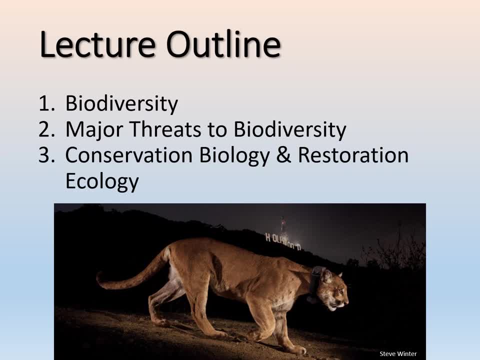 increased biodiversity and decreased biodiversity, as well as what are some of the major threats to biodiversity right now, But also why is biodiversity important, or why is it good to have biodiversity, And then what can we do to combat those threats to biodiversity? and that's really where conservation biology. 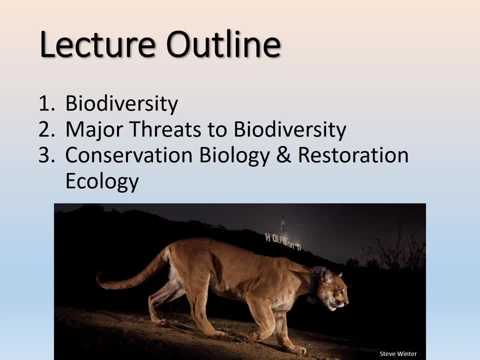 comes into play as well as restoration, ecology, Right. so this is a great picture of a mountain lion near the Hollywood sign, because we see mountain lions a lot these days and their space is crossing over with our space, right, So this is where it affects us, right, every day, when. 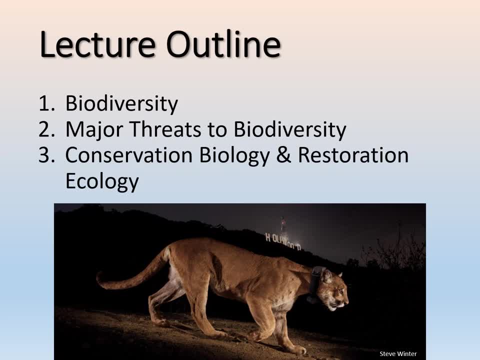 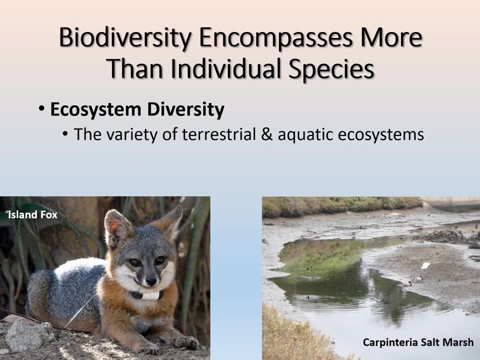 we see wildlife in our backyards and what can we do about that and what should we do about that, maybe? So when we're talking about biodiversity, we're really talking about more than just the species level and the individual species, So really we're talking about more ecosystem. 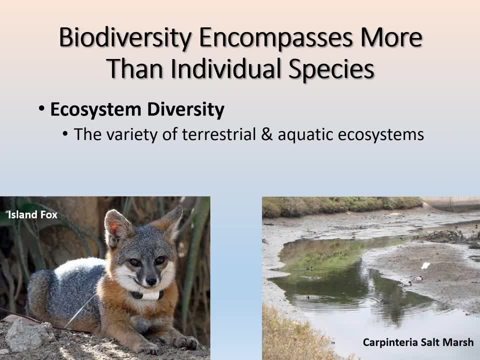 diversity and the variety of different species that we see in the terrestrial and aquatic ecosystems. So we have talked a bit about the island fox out in Channel Islands and what happened to them. We started out as the very special Carpentry of salt marsh where we have a lot of very rare 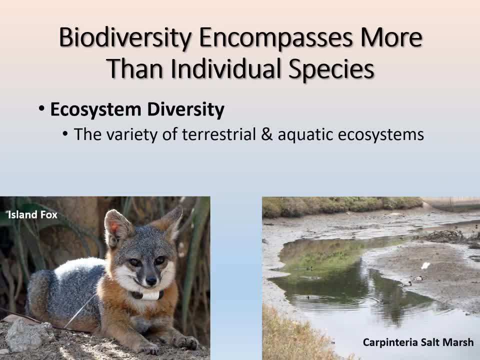 species and a lot of biodiversity seen in the salt marsh. So really we have some of these very rare ecosystems around the world and we're lucky to be kind of near a lot of them, including that salt marsh, But just the chaparral as well. that. 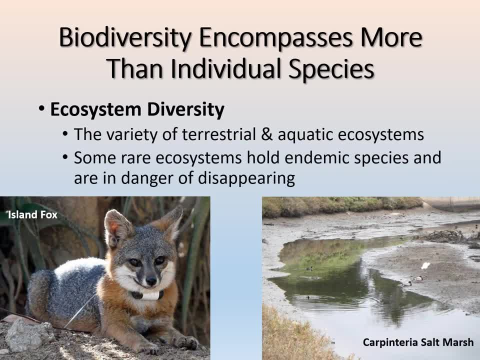 biome that we live in holds a lot of endemic species, meaning they only live in these ecosystems and really when we talk about these you know rare endemic species. they can be in danger of disappearing if we don't worry about biodiversity and kind of taking care of those ecosystems and combating those. 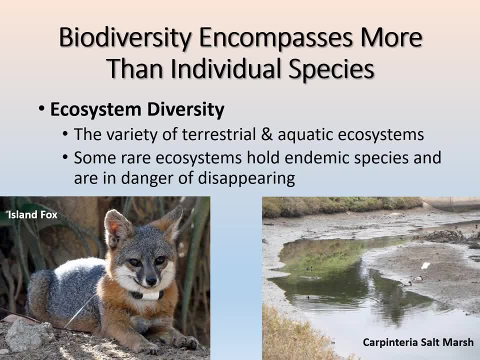 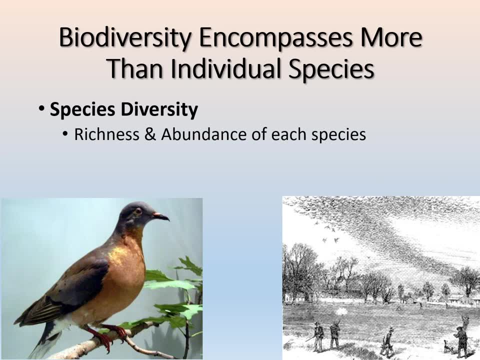 threats to biodiversity. that we'll talk about. so that was ecosystem diversity, but we can also talk about species diversity, and so that's at the species level, and you're talking about the richness and abundance of each of these species in these different ecosystems. so when we're talking about a species in a 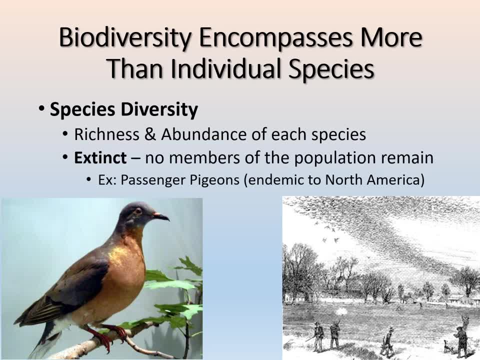 population. you can tell about what species a population is, but when you get to talked about each of several species, environmental choices and population, the energy efficiency is potentially treat expanses from different species and peoples- you can talk about extinction right. So if we talk about extinction, that means that no members of the 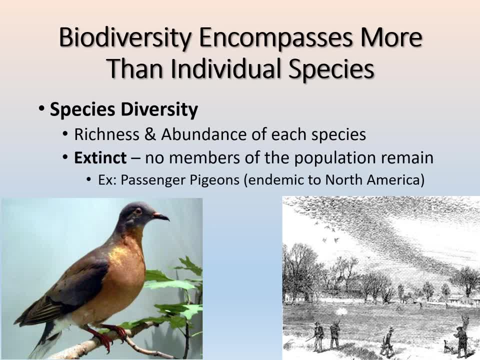 population remain of that species right. So, for example, we have the passenger pigeons that were endemic to North America, meaning they were only found in North America And they used to be the most numerous bird in America And they would fly in these massive flocks almost a mile wide and 300. 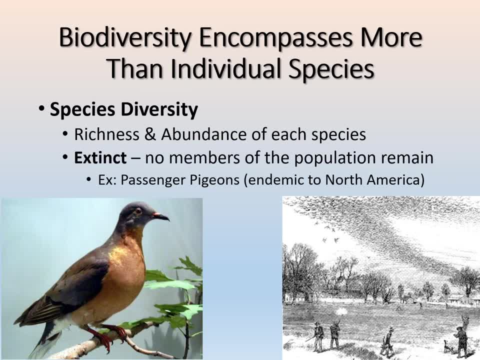 miles long, where it would actually take almost 14 hours for a for one flock to just pass over and fly overhead. That means there was close to like 3.5 billion birds. That's a lot of birds, But of course you know hunting definitely. 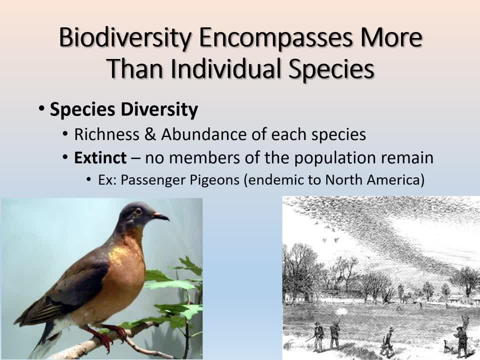 took them out, And there was a final flock in the late 1800s where there was only about 250,000, or about a quarter million left, And they were actually killed by one group of hunters who knew that they were the last flock in existence And they essentially did not leave any bird behind. 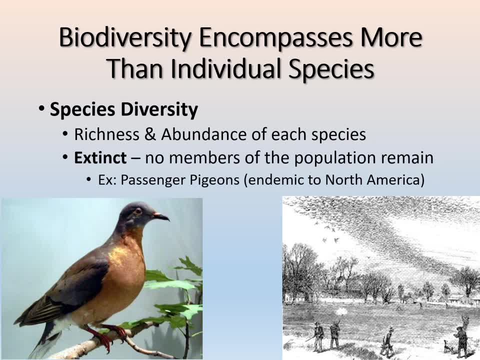 which is really crazy, that these hunters actually took out all these birds. So basically, they were the last flock in existence And they essentially did not leave any bird behind, which is really crazy that these hunters actually took out all these birds. Soophallia is one of the 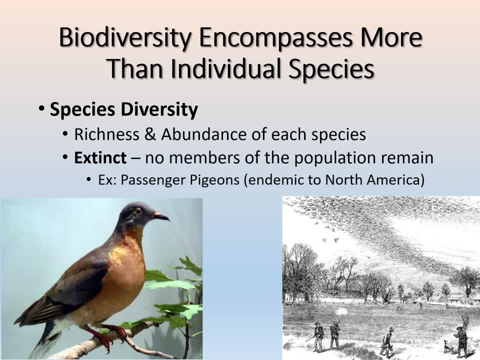 very sad, but there is no longer passenger pigeons in the world and they were endemic to North America and they were a social bird, so they used to nest in groups and so I think they just their numbers got too low to be able to survive just individually, since they were such 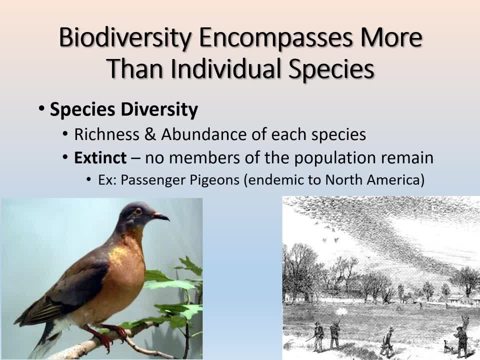 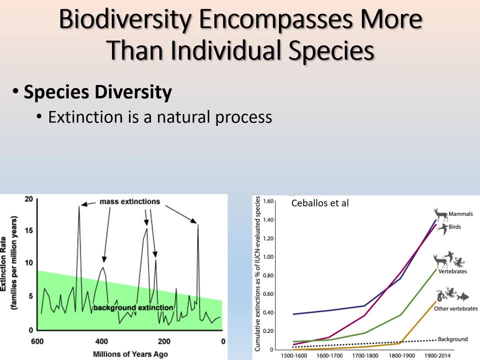 social birds, so they are considered extinct now. So when we talk about extinction it's a very natural process. so we may think that extinctions are very rare and maybe they're only happening right now, but in the fossil records they actually. 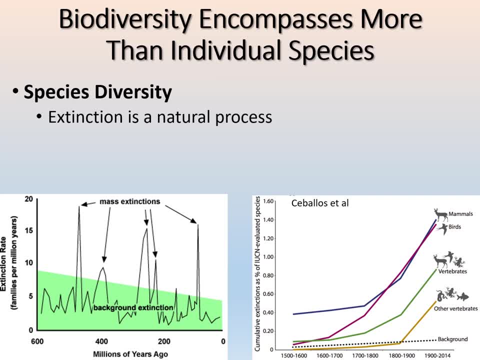 show these very slow extinction rates. so if you look back and our one table here shows about over 600 million years ago, you notice that there are extinctions that are fluctuating and we call that background extinction, And so that's just kind of slow extinction rates that are happening all the time. right, they're just 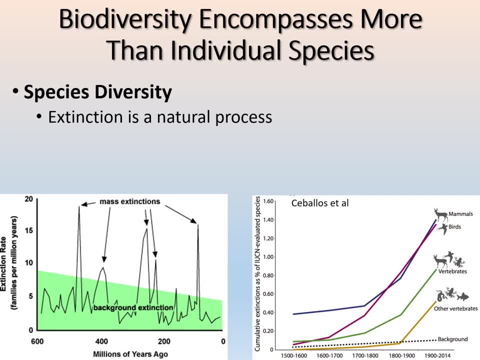 always occurring. but then we have these spikes in the extinction rates and we call those mass extinctions. and so we have had five mass extinctions over kind of the fossil records and we're currently considered to be in the sixth mass extinction. 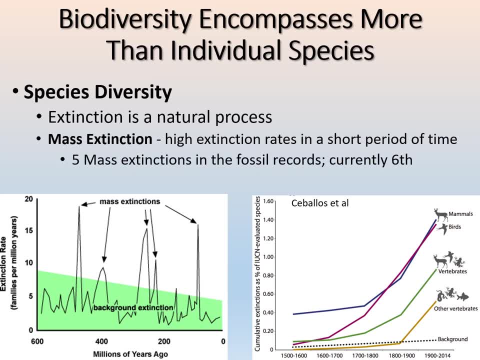 And so that's just kind of slow extinction rates that are happening all the time. but then we have, And that's really due to humans. So we talked a lot about human population and how it's driving extinction of other species And so really the last extinction was about 65 million years ago when the dinosaurs went extinct. 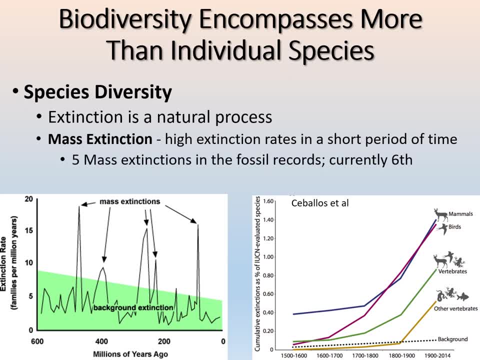 But now we're really into this sixth mass extinction, And usually mass extinctions are due to rapid climate change- meteorites, things like that, that have a very strong effect either to the climate and to these ecosystems, And so we're losing other species, right. 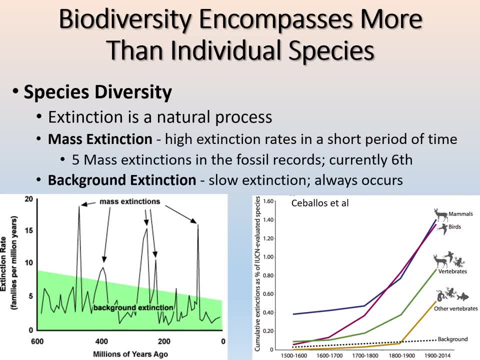 So if you look at the graph on the right, it's showing kind of these cumulative extinctions as a percent Of kind of all the evaluated species And if you notice we have a very severe increase in kind of all vertebrates since the 1900s, but specifically mammals and birds. 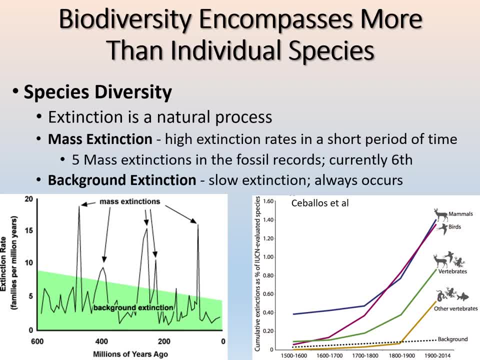 So birds are definitely up there with extinctions And when you talk about kind of natural extinction rates of birds, you're talking about one every maybe 400 years. you have an extinction of a bird species, But lately We're getting one every year for the past 500 years due to humans. 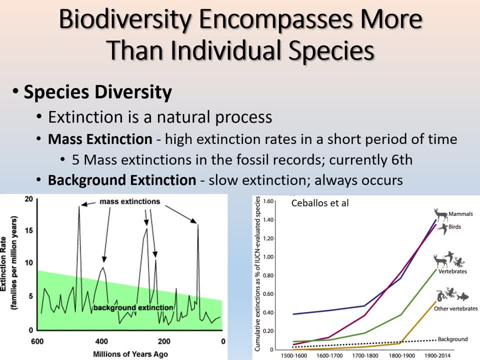 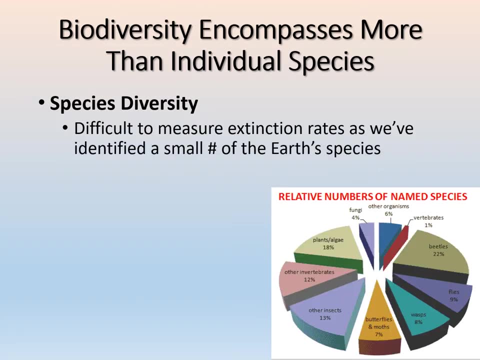 So we have definitely increased the bird extinction rate significantly, as well as mammals and other vertebrates as well, as you can see on the graph. So we have these graphs and things that are kind of very subjective. It's really hard to measure extinction rates really accurately. 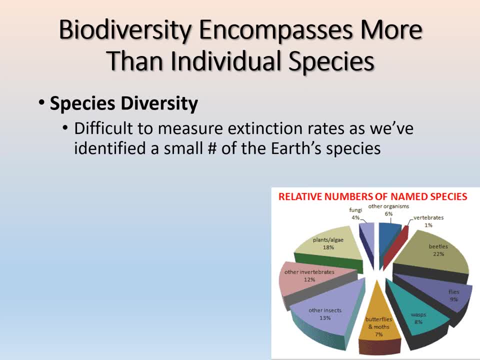 So this is kind of the data that we have, because we haven't even identified all of the earth species period right. We've only identified a very small number of the earth species. So we actually have estimated that there's about 8.7 million species on the earth and we've only identified and named 1.9 species. 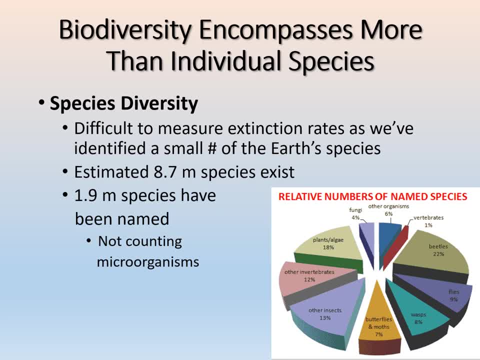 So that's not even counting micro organisms, right? So all the bacteria and parasites, all those microorganisms we're not even counting in this number. So that is just a crazy amount of species to even discover, right? So how can we be that accurate when we don't even know all of the species that exist on earth? 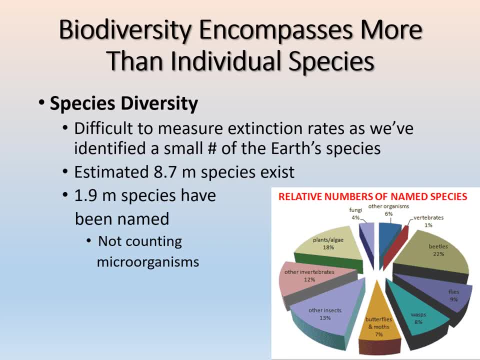 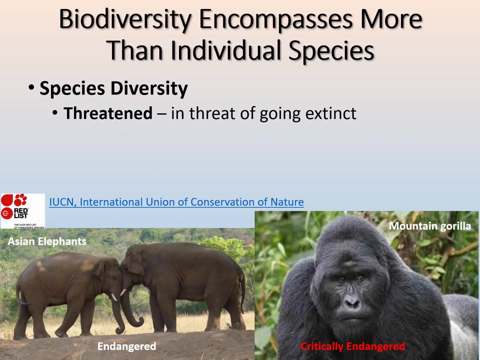 So So again, very hard to measure these extinction rates. We're just working with the numbers that we have and it's probably fairly representative of the Earth species, But again, we just don't know, right. So when we're talking about extinction, we have some levels of species diversity coming before extinction, right? 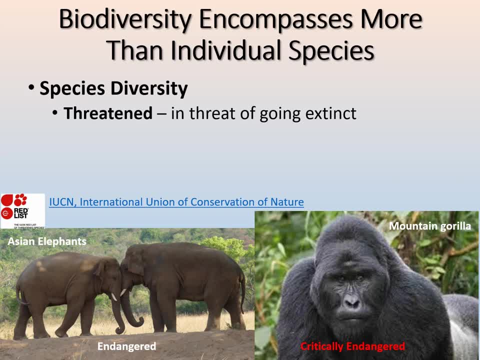 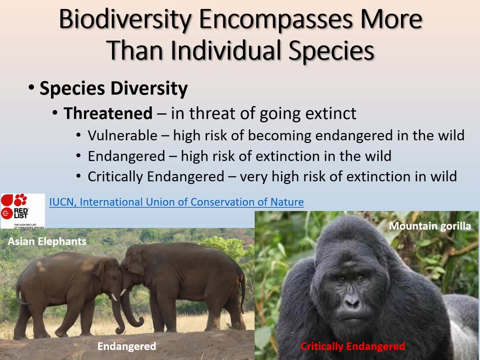 So we have species that are threatened, meaning they're in threat of going extinct at some point if the numbers continue the way they're going. So what are these threatened species that are not necessarily extinct? And so we have some different categories And, if you're interested, there's a conservation, the International Union of Conservation of Nature, that actually keeps track of all of the species and where they are on this threatened list. 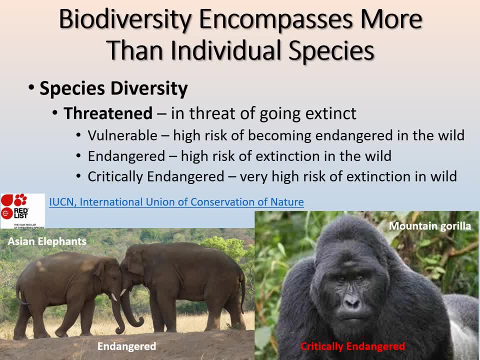 And they call it the red list. So that's the red list. meaning where are they on the threatened list, right? So are they vulnerable, meaning they're at high risk of becoming endangered in the wild. So then, what is endangered? Well, endangered is at high risk of extinction in the wild, right? 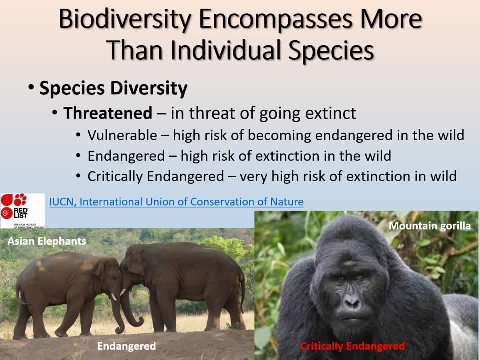 And then critically endangered, meaning a very high risk of extinction in the wild. So again, we're talking about the wild and not necessarily captivity, right, Because animals in captivity- a lot of them- are trying to combat These threatened species. So, if you look, just two examples that we have and maybe you've heard of right are the Asian elephants are endangered. 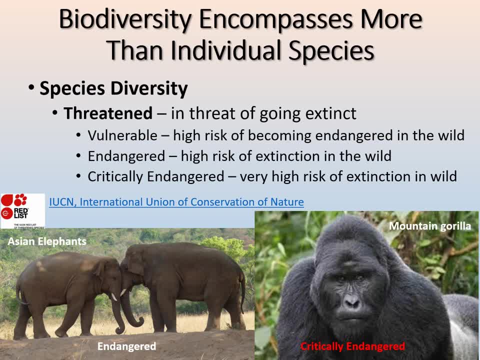 So they're at high risk of extinction. but the mountain gorilla are critically endangered, meaning they're at very high risk of extinction. So if you're interested in that, go ahead and check out the link and I will put the link on canvas as well for you guys. 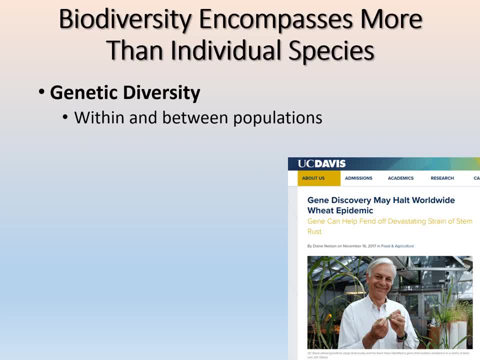 So we've talked about ecosystem diversity, species diversity, and now we can talk a little bit about genetic diversity. Genetic diversity is something we have kind of touched on before right, Which with genetic variation and things like that within and between populations. What is that genetic diversity? 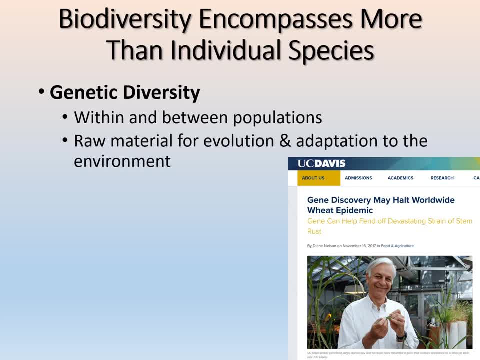 So this is really kind of the raw material for evolution and adaptation, Right? Yeah, So if we have genetic diversity and variation, then we can have selection and adaption or adaptation with those mutations and things like that to the environment and therefore hopefully continue a population, right? 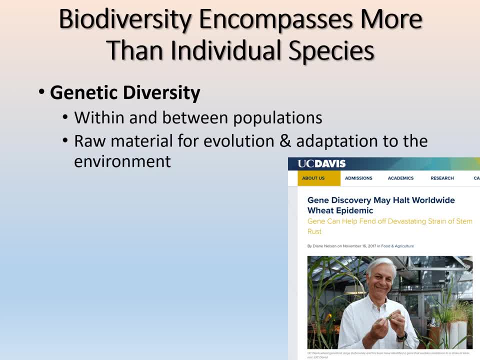 The population can survive. So that's really the importance of genetic diversity. But there's some interesting things with genetic diversity, Especially for crops, as well. So obviously we talk about genetic diversity within humans and within, you know, animals and things like that. 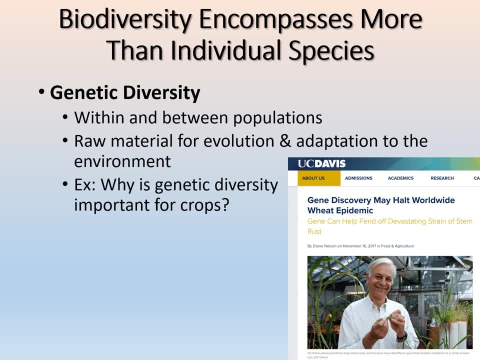 But again, there's some great importance for crops to have genetic diversity, And so this example I have here out of UC Davis is that there was a there's a new fungus essentially out there that's wiping out the weeds Right, And so there's actually a resistant gene to that fungus that they found in a relative of the wheat that's over there. 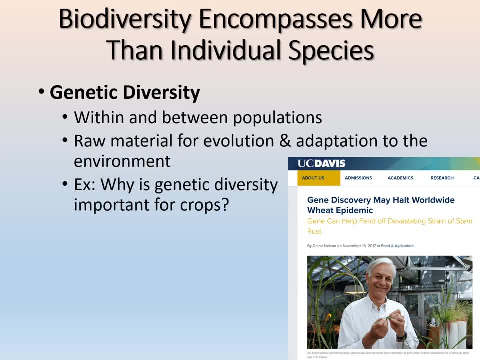 And so either they can switch to this relative wheat species and start growing that, or they can use genetic engineering to study and possibly transfer the genes from this relative to the current species out there. So essentially, this specific resistant gene could help fend off that fungus that's causing such devastation over there. 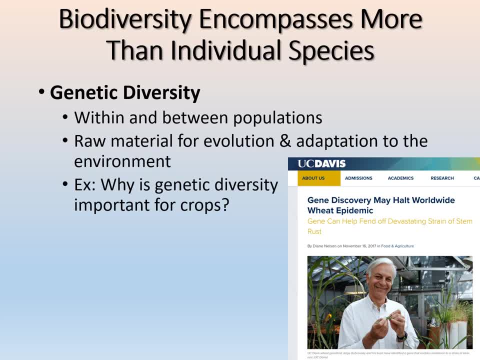 So this may hold the key to kind of the world's future food supply, right. So we need to maintain that genetic diversity within crops, within species, within populations, right. We need to have that genetic diversity To continue the survival of that species and of that population especially. 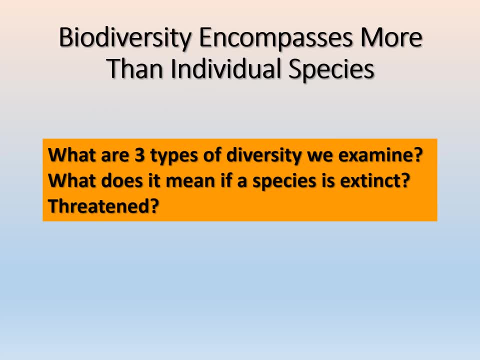 So let's pause the video and have a little bit of review. So what were those three types of diversity that we just discussed, And what does it mean if a species is extinct versus threatened Right, What's the difference? So hopefully you guys were able to pause the video and go through that. 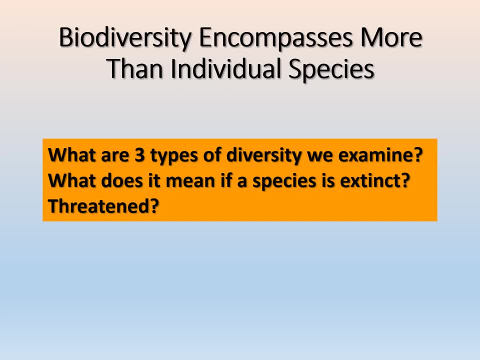 Should be fairly straightforward. We talked about ecosystem diversity, Right. We talked about species diversity, And then we talked about genetic diversity, which is one we've kind of discussed before, Right. And so if a species is extinct, That means there are no individuals left of that population or of that species. 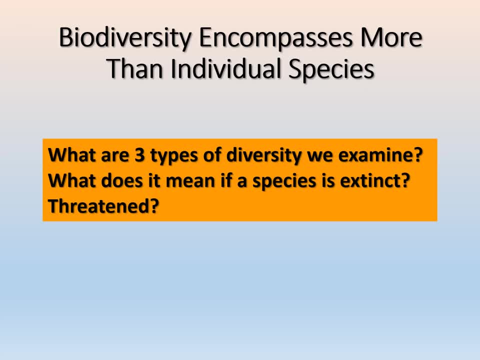 Right. And then if it's threatened, we talked about kind of the different levels of threatened Right: Vulnerable, endangered and critically endangered Meaning that they have a certain level of risk of becoming extinct in the wild Right. So that's the difference between extinct and threatened. 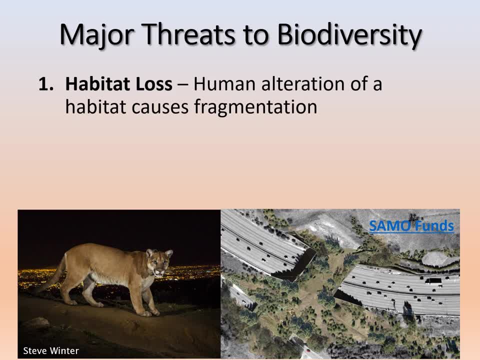 So now that we know a little bit more about biodiversity and what it means and why it's important, not only at the genetic species but also ecosystem level right To have all this biodiversity. So what are our major threats to biodiversity? What's happening right now that maybe we can change or do something about to stop? 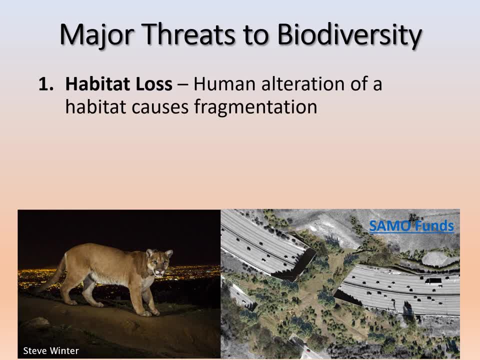 The decrease of biodiversity. So our first major threat is habitat loss. So this is definitely something we see in our area but all over the world, And that's human alteration of a natural habitat, causing this fragmentation of their habitat. So a species is going to have a certain area of land. 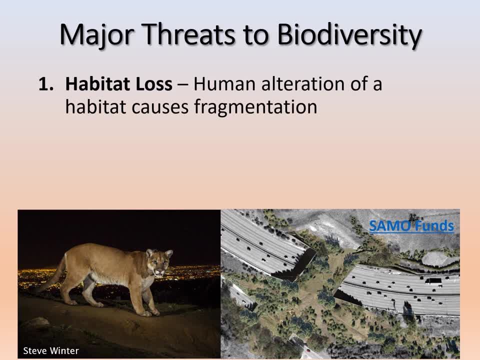 Right, That considered its habitat And that's where it roams and lives and finds its resources for survival. So what do we do? Well, things like agriculture, urban development, forestry, mining, pollution- all of these things are going to aid in habitat loss. 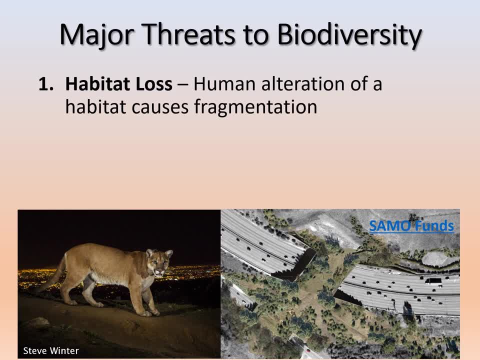 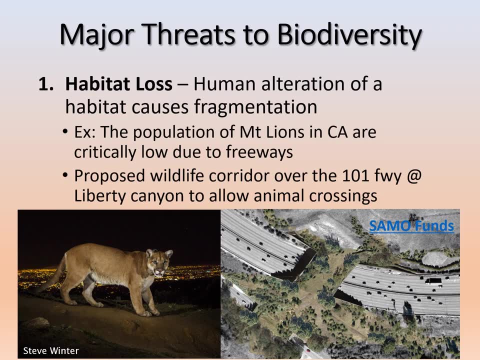 Right, So these are all human alterations of habitat. So, for example, We've been talking a little bit about the mountain lions in California And the populations of mountain lions are actually critically low, And a huge cause of this is due to freeways. 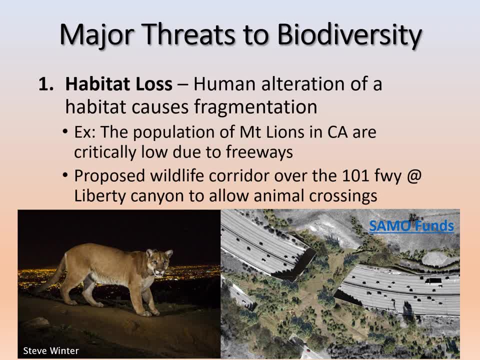 So freeways are essentially causing a fragmentation of their environment. So they're trying to cross freeways and they're getting hit, And so they're proposing these wildlife corridors, Well, all over, But especially over here Off the 101 freeway at Liberty Canyon, to allow animals to actually cross the freeway safely in a more natural environment. 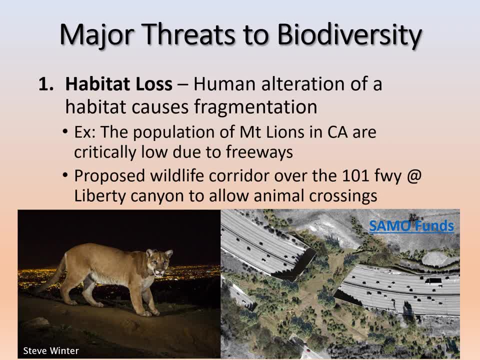 And what I'll do is I'm actually going to link a video of a natural corridor that's actually functioning very well in another part of the country, And so we're hoping that maybe we can emanate that and do that over here as well. 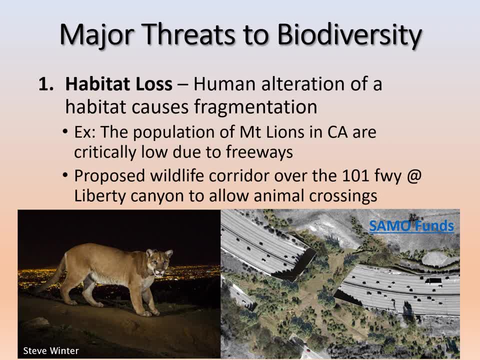 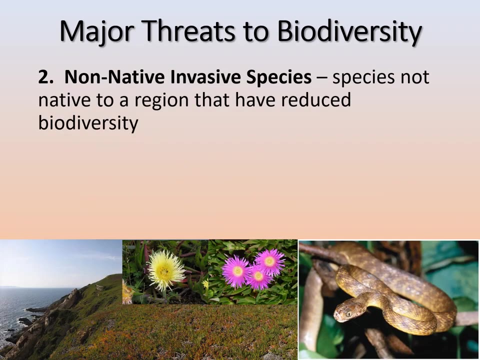 So it has been proven to work And these SAMO funds are essentially funding to try to get this project to come through and actually get built. Okay, So you can check that link out as well if you're interested in the project. So another major threat to biodiversity are those non-native species. 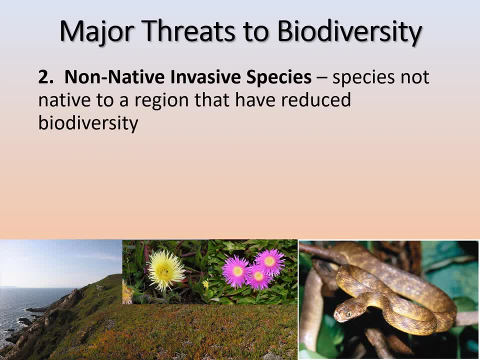 So these are species that are not native to a region and they have been introduced, whether by humans or accidental introduction. So usually they're humanly human introduced, But again they could maybe be carried by something or something like that, But these guys have been introduced to a region. 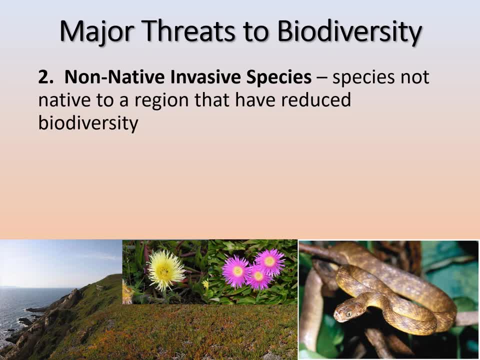 They're not native to And they essentially reduce the biodiversity in that area because they lack the environmental resistance of that area. They didn't, they didn't evolve in that region, So they do not have the interspecific competition. Maybe they lack predation. 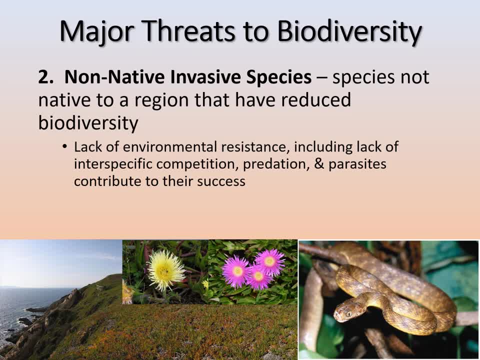 Right, And maybe they lack the parasites of the area, And so all of these, in these environmental resistances that they are able to overcome, contribute to their success. So some examples that we've seen, or you know just other examples. we've talked quite a bit about invasive species. 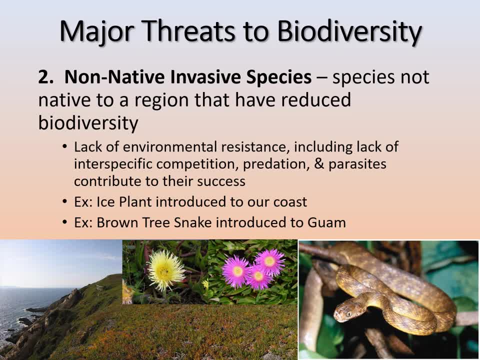 But in our area, on our coast, we have a non-native ice plant. So if you notice, you know a lot of the coastal lines are covered With this ice plant And it's actually not native, So it's just taking over. 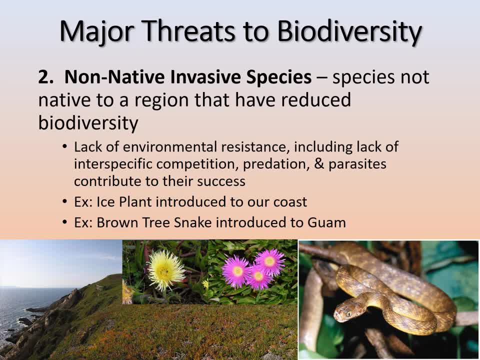 And it's decreasing the biodiversity and pushing out all of the native species of the area, As well as this brown tree snake that was introduced to Guam. So they're native to kind of coastal Australia, eastern Indonesia area, And so they were actually brought over. 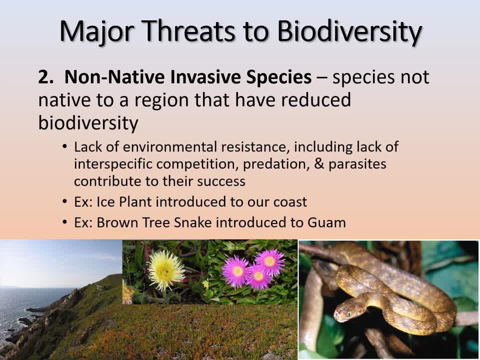 In a cargo plane in the 1950s to Guam And now they have caused a lot of extinction of the natural and native populations of Guam. So there's usually about 13 species of forest birds out there And when the snake was introduced three of the bird species are now extinct. 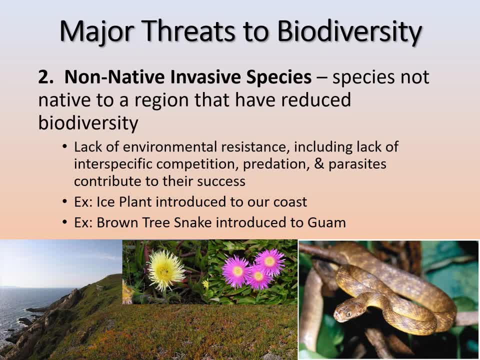 Four populations in the island are extinct, But they're found on nearby islands, So essentially they have moved off the island and gone elsewhere because of this snake, And now there's, you know, more than 20 snakes in every acre of land. 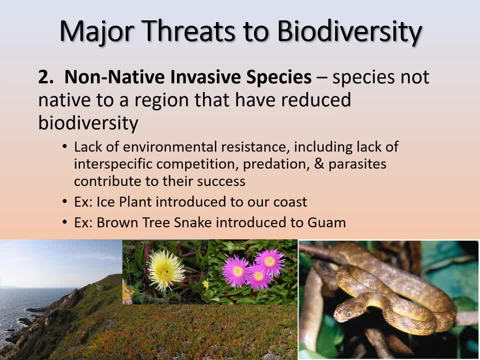 So that's you know. they're definitely just going crazy, right? They're pushing out all the other native species And they're causing extinction of other species, So they're greatly decreasing The biodiversity. And that's fairly easy to do in an island setting, right. 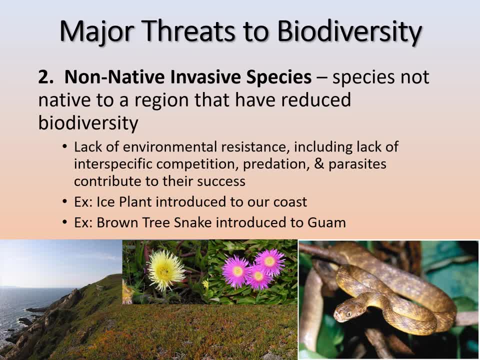 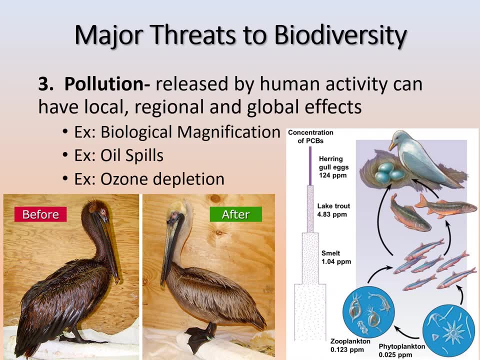 So islands are very susceptible to quick change in biodiversity. So another major threat to biodiversity, which is fairly common, right, is pollution. It's something that we all know about And this is definitely caused by human activity And it can have very local, regional and global effects, right. 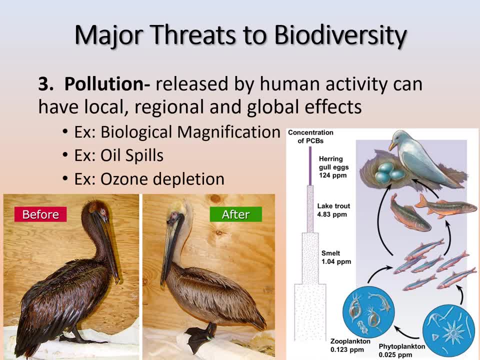 So there's a couple examples of pollution. A lot of people know about oil spills, right? So oil spills in the ocean causing detriment to the marine wildlife, right? This poor pelican covered in oil before and after being cleaned, So that's kind of one we definitely know about, right. 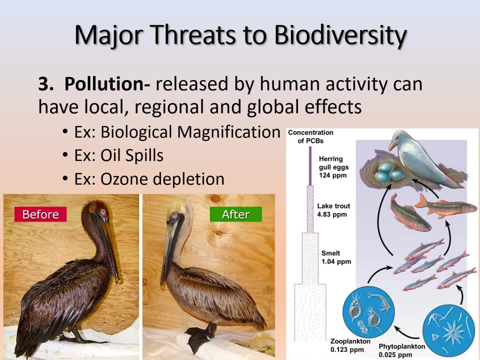 And then we have what's called biological magnification, Meaning that there is transfer of these pollutants from terrestrial to aquatic ecosystems, right? So you're releasing all these chemicals into the environment And they're going to move up the trophic levels, right? 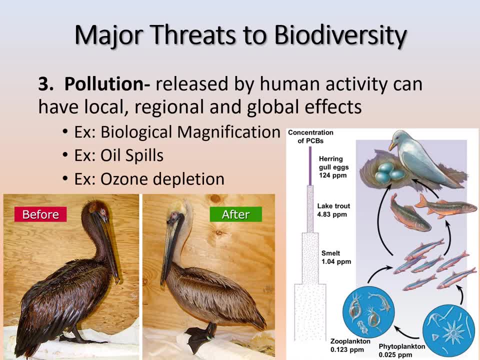 So we talked about trophic feeding levels And what happens is is that the chemical is going to get more and more concentrated as we increase or go up the food chain up the trophic level. So you know, DDT was an example of that. 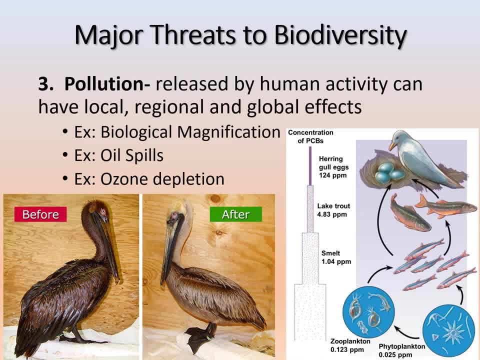 But also these PCBs, And they are. what happens is it just keeps increasing up the levels Right Up the level of the food chain. So these high food chain level individuals and animals are getting hit very hard due to this biomagnification. 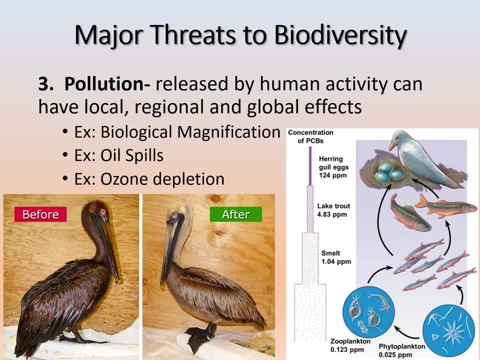 And another one is the ozone depletion. right, So we're releasing these chemicals that thin out the ozone layer, And the ozone layer is what protects the earth from UV rays- right, So these harmful chemicals, So these harmful UV rays, are going to increase problems such as skin cancer and all kinds of other things as well, right? 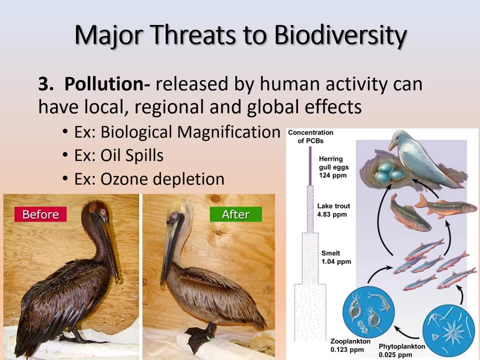 So we kind of know about that too, And the release of carbon dioxide and things like that into the environment. So lots of pollution going on. that we kind of all know about. right, We know it's happening And we know that it has a lot of detrimental effects on the environment. 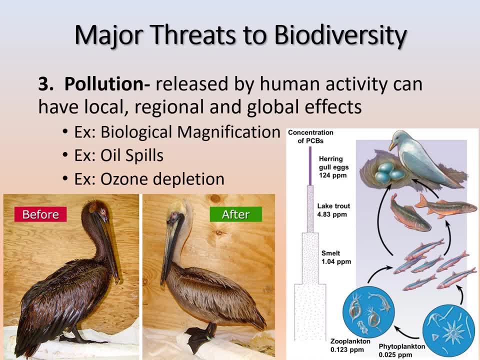 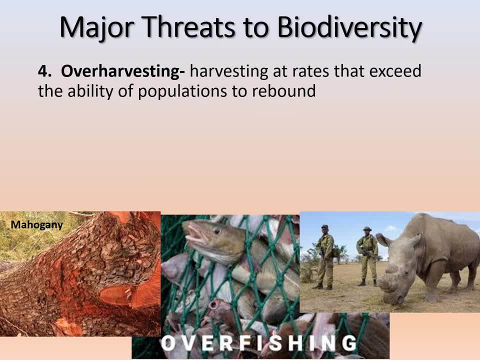 But also to biodiversity. So another thing caused by humans as well. Another major threat to biodiversity is over-harvesting. So essentially any kind of harvesting that's at a rate that exceeds the ability of that population to rebound or recover. Okay, 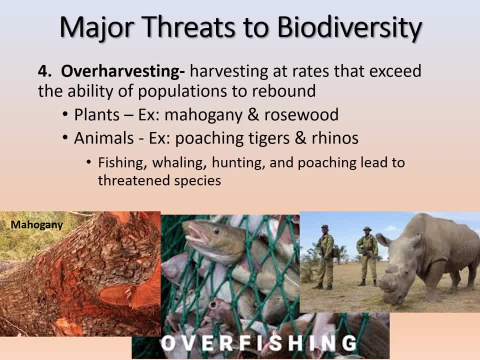 So this could include plants and animals right. So any sort of fishing, whaling, Hunting, poaching, Foresting, right, Deforesting- So all of that is considered- can be considered over-harvesting if it's at a rate that exceeds a population's ability to recover. 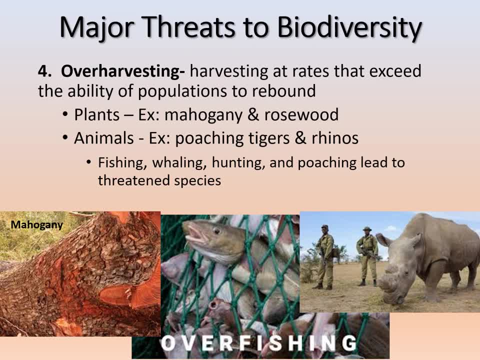 So we've seen that with mahogany and rosewood trees. So that's an example in plants, But we also see it with tigers and rhinos, With poaching right. So over-fishing, over-whaling, hunting, All of this can lead to threatened species if that species is unable to rebound from that over-harvesting. 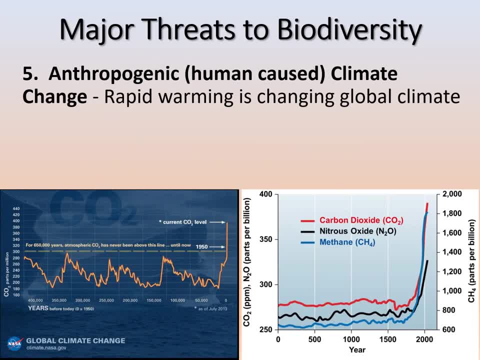 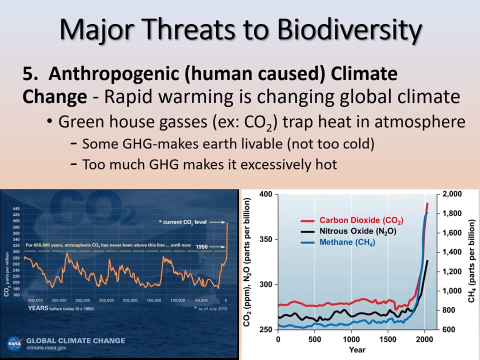 So our last major threat we're going to talk about to biodiversity is anthropogenic, meaning human-caused- climate change, And that is a rapid warming of the global climate. Okay, So that means that our global climate is increasing in temperature, And so if we talk about greenhouse gases, greenhouse gases- an example of a greenhouse gas- is carbon dioxide. 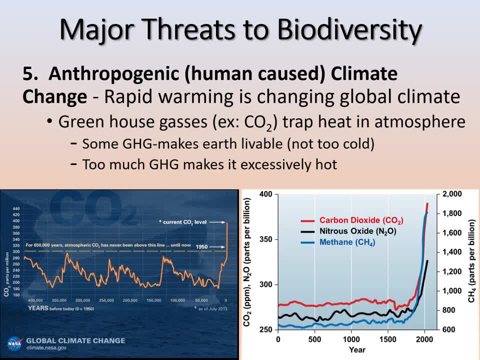 But we do have other greenhouse gases as well, But the main one a lot of people talk about is carbon dioxide, And carbon dioxide, or greenhouse gases, are important because they trap heat in the atmosphere And they're good to a certain degree, because some greenhouse gases make the earth livable or viable. right, 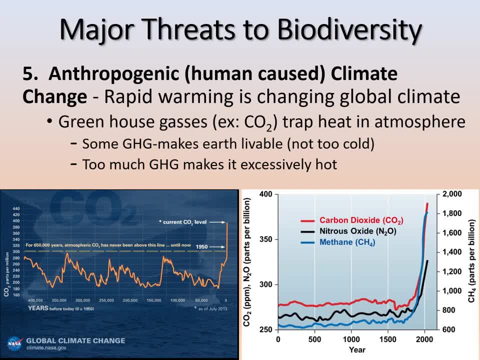 So that the earth is not too hot. So we do need a certain amount of greenhouse gases to actually survive. But too much greenhouse gas and it makes it excessively hot, right? So if you trap too much heat in the atmosphere, you're going to increase the overall climate. 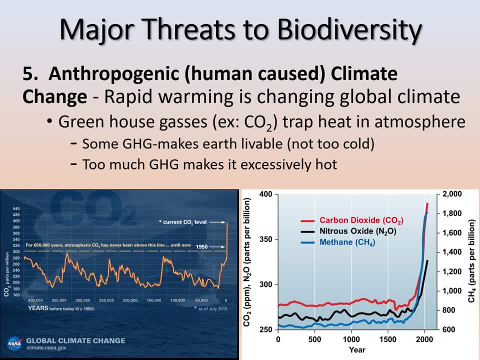 And so, if you notice, you know this has been a controversial topic. you know, among the general public is the global climate change, But it's not controversial among scientists And for some reason, you know, graphs and data just can't convince the general public that something is happening. 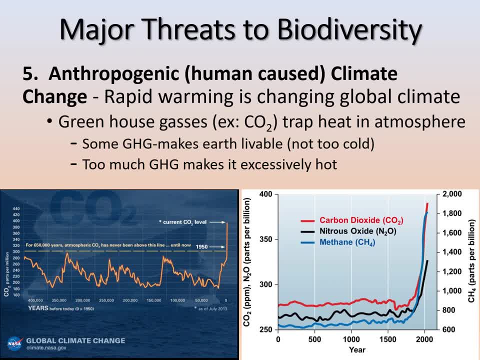 So you know a little bit on my soapbox there, But in the scientific world this is not something that should be controversial, It's just a fact. But regardless, right? So we see that we have the highest CO2 concentrations since about 600 years ago. 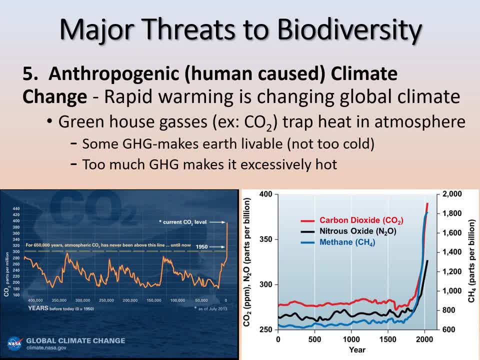 About 650,000 years ago. Okay, So we've seen kind of this highest plateau of about you know, 300 on that graph, that brown line, And obviously we have, you know, this cyclical increase and decrease of CO2 in the atmosphere. 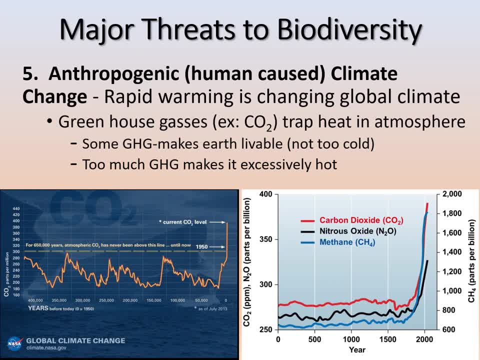 That just makes sense over history, But it's the highest it has ever been in this recorded history Here. So that is telling you something, that something is going on right. We have excessive carbon dioxide and greenhouse gases, And so same with our graph on the right hand side. 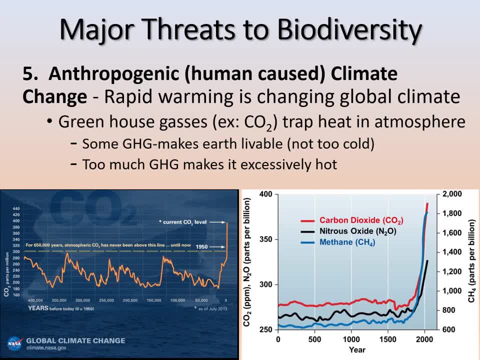 You see this kind of cyclical pattern with carbon dioxide and all these other gases in the environment, And then you see kind of this steep, steep increase towards carbon dioxide Towards approaching the 2000 year, right, So the bottom axis is years. 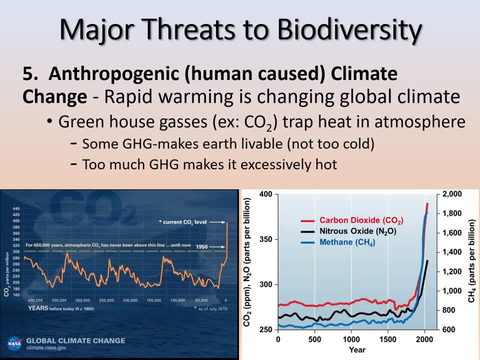 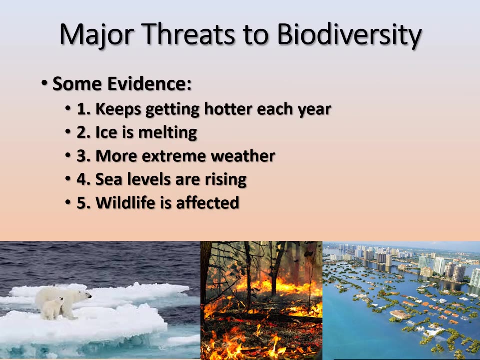 And then the y-axis are the CO2 and methane in parts per million. So we see this rapid increase, And so you know we are blaming humans for this rapid climate change and increase in climate change, right? So what are some evidence for this? you know, global climate change. 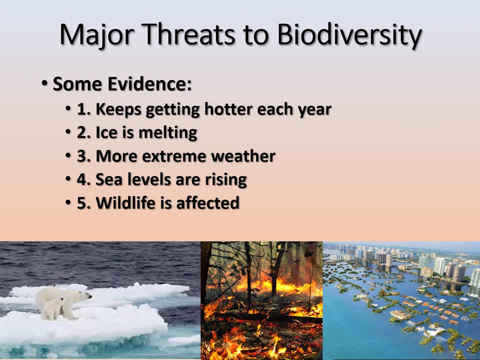 And we see that it keeps getting hotter each year. right. So we have this increased temperature climate. We know that the ice, the polar ice, is melting. right, Which is threatening a lot of species up in the polar regions. We have more extreme weather, right. 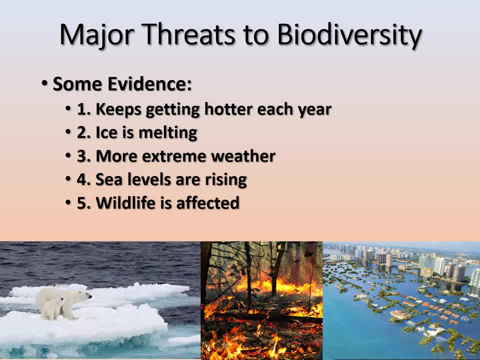 We're seeing that We have more hurricanes, more fire, things like that that can be contributed to weather. The sea levels are rising because the ice is melting- right. We're adding more water to the sea levels and the wildlife is being affected, right. 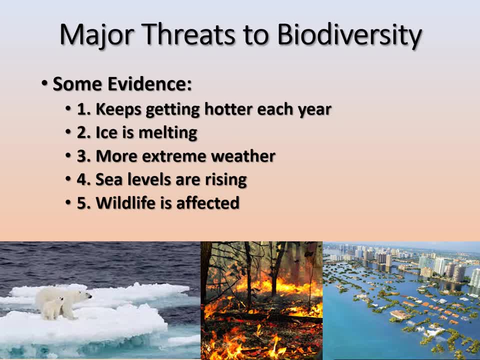 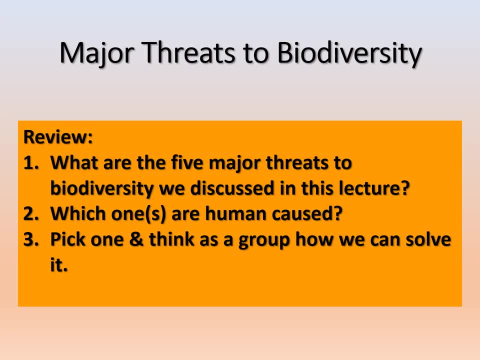 So these are all kind of some evidence for this global warming. So let's pause the video, right, So you can do a little review. What are the five major threats to biodiversity that we discussed in this lecture, right? So obviously there's a lot of threats to biodiversity, but we discussed a few of them. 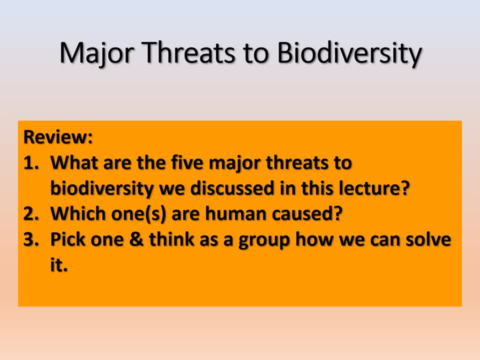 Which ones of those are caused by humans, right? And then obviously we're not in lecture, But if you want to pick one, But if you want to pick one and think you know to yourself, how can we maybe solve it right? 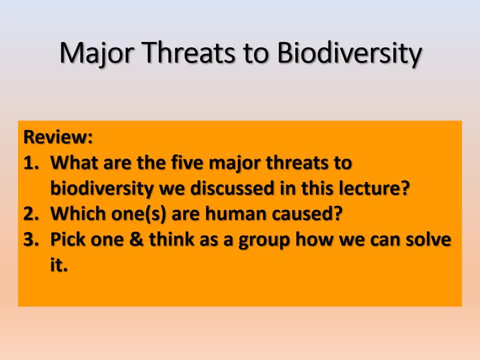 What could be something that we could do about this threat to biodiversity? What could we change to help it right? So go ahead and pause the video and look through that. We won't go through it just because you know it's pretty easy to look back through that, okay. 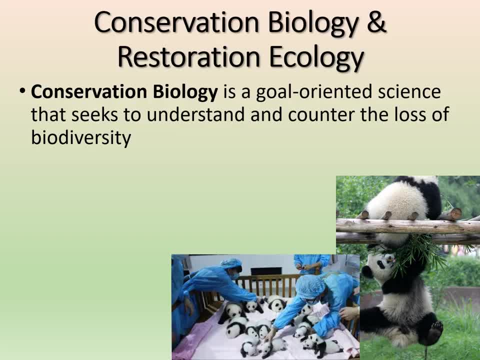 So now that we know the threats to our biodiversity, how can we maybe combat those threats? And that's called conservation biology. So it's really a goal-oriented science And you're trying to understand and counteract that loss of biodiversity. But you need to understand a couple of things when you're doing conservation biology. 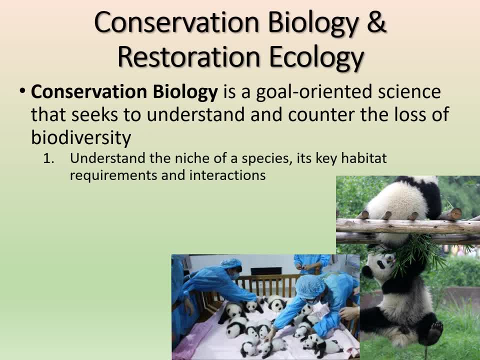 So you have to understand the niche of that science, The niche of that species. So where is their key habitat, What are the requirements of that habitat for that species And what are their interactions, not only with other species, but also with humans as well, if humans are, you know, the main threat to biodiversity? 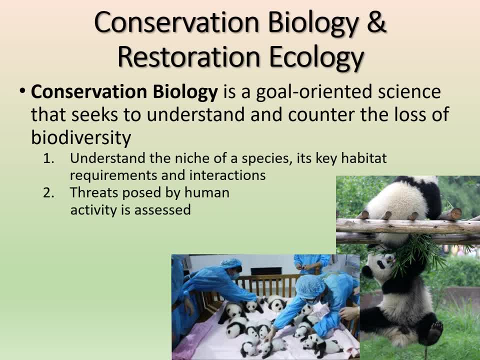 So you really have to know what those threats are that are posed by human activity. So you have to assess that, So you have to assess that situation. So is it deforestation, Is it hunting, Pollution, Whatever that may be, that's causing the threat to the biodiversity? 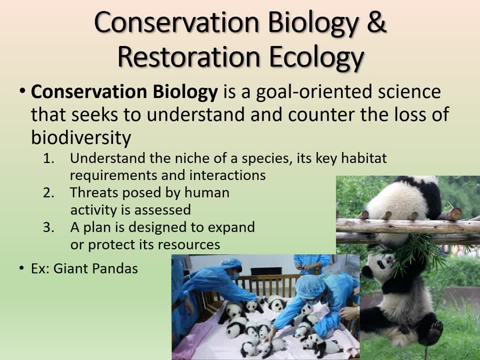 And then you have to make a plan right. So you have to design a plan that's going to help expand and protect the resources for that species in that habitat. So, for example, I'm sure many of you guys have heard about the giant pandas over in China. 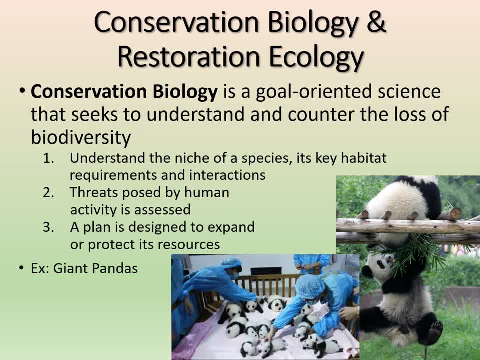 And they were on the endangered list right. So there's been poaching and logging of their bamboo habitats since the 1960s And they put a ban on logging of the bamboo in about 1998.. So not too long ago. 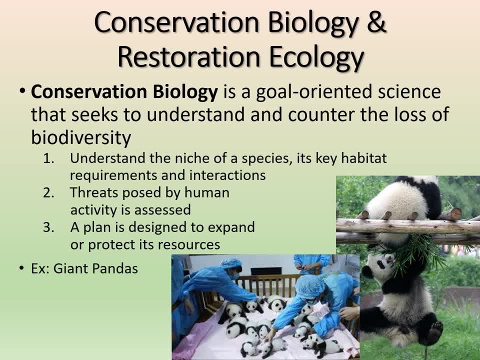 And they essentially made these nature cores Between the reserves, between the nature reserves, And they started captive breeding programs to help increase the numbers of the giant pandas. Now you can imagine, obviously giant pandas are quite cute, right? So they were able to really do a lot of PR for the giant pandas and really raise a lot of money for this program. 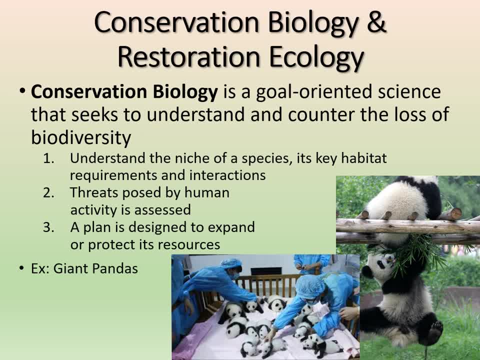 So it was really interesting, So it was really a very successful program and they're no longer endangered. But if you research a little bit about the giant pandas and the programs and how the Chinese kind of use them as PR statements and political statements, then there's a whole kind of can of worms there with the giant pandas. 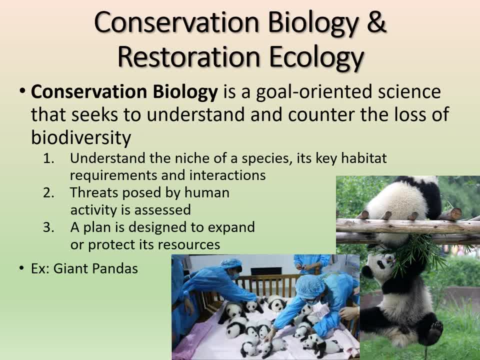 But again, right, they're cute and cuddly and everybody wants to help save them. But what about all those endangered species? There are some endangered species that maybe nobody knows about, Nobody cares about. They're not cute and cuddly And you can't really raise the kind of awareness in the public eye as you can for some of these other species that people really kind of care about. 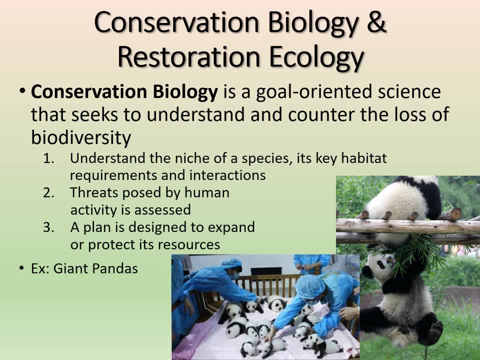 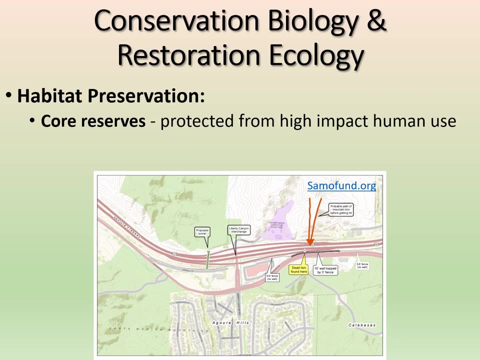 So just something to think about when you're talking about conservation biology as a whole. right, What kind of species are people trying to help? So what are some of the big goals of conservation biology? So we want to do habitat preservation, right. 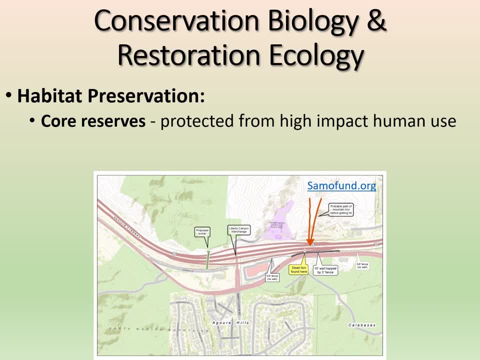 So we want to have these core reserves to protect these habitats that the species live in, And so what happens is is they're protected from high impact human use. So essentially, they ban things like logging or hunting or things like that, so that we have this core reserve for that species. 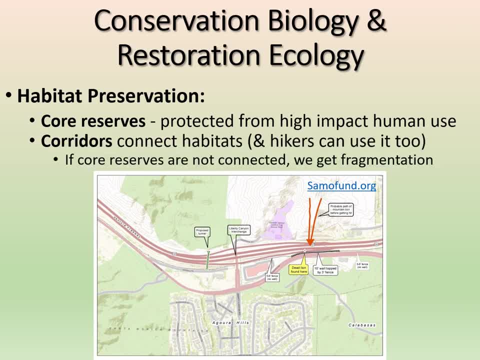 But then again you may have this fragmentation that happens where their habitat is split up right. So in those cases you want to make corridors that are going to connect those habitats that the animals and even hikers can use them to. So you know, if these core reserves are not connected, they get this fragmentation and that can definitely be detrimental. 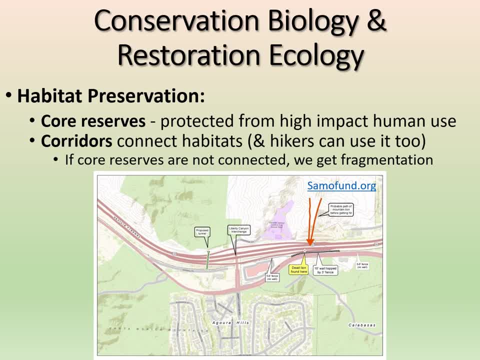 So we talked a little bit about the mountain lions. We talked a little bit about the mountain lions in Southern California, in the Santa Monica Mountains. So that's really kind of what's happening just kind of in our backyard right. So again you can see what's happening just in our own area and what they're trying to do about it and create those corridors for the mountain lions in kind of the Agora Calabasas area. 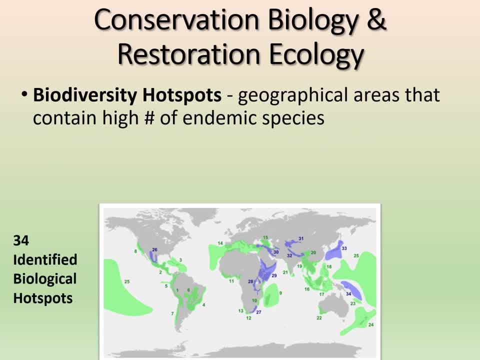 Okay, Okay, Okay, Okay. So another way that conservation biology tries to help, you know, maintain biodiversity and restore biodiversity is focusing all of their efforts on these biodiversity hotspots. And what are these hotspots? They're actually geographical locations that contain a high number of those endemic species, meaning that they 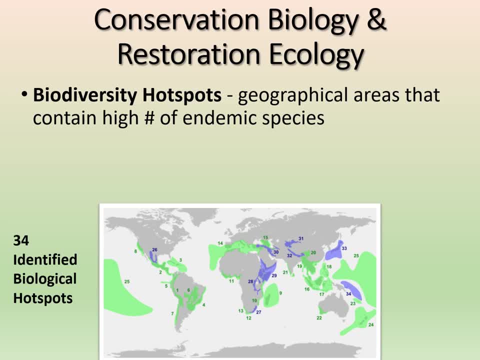 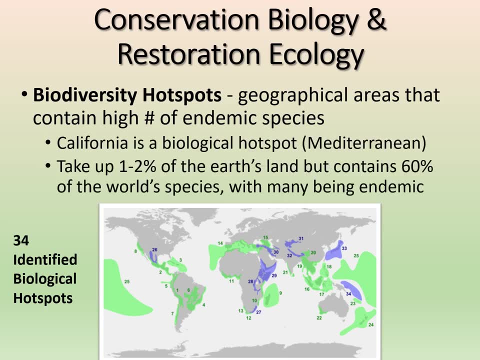 These species only live in that kind of environment, that kind of habitat, that kind of biome, right? So we've seen that word endemic species before. So take California, for example. we are a biological hotspot. So we talked about that chaparral or Mediterranean biome being kind of very important for endemic species and being kind of this biological hotspot. 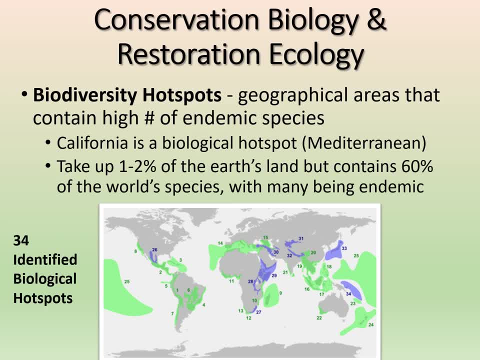 So if you notice, kind of looking at the map here we have 34 kind of identified biological hotspots. A lot of places make sense right, Like Brazil, Costa Rica, Central America, you know, the Pacific Islands, things like that, even the ocean right. 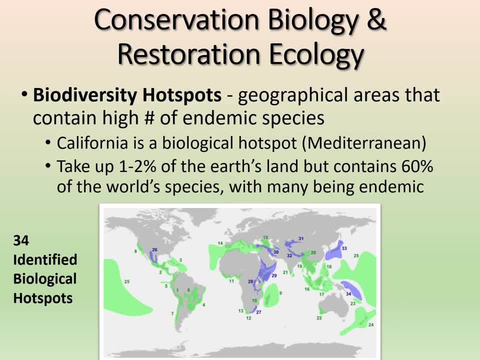 So the Pacific Ocean, Mediterranean, so New Zealand, kind of all these places that they take up only about one to 2% of the population, The Earth's land, but they contain 60% of the world's species. So that means over half of, you know, the species that we've identified anyways. 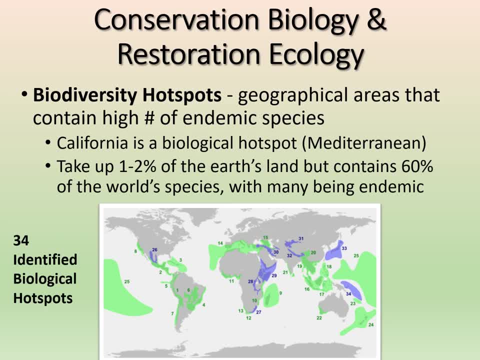 And many of those species are endemic, meaning they only live in that environment. So if you can focus kind of your energy and resources to these biodiversity hotspots, you have a better chance of, you know, keeping or maintaining or even restoring the biodiversity in those regions. 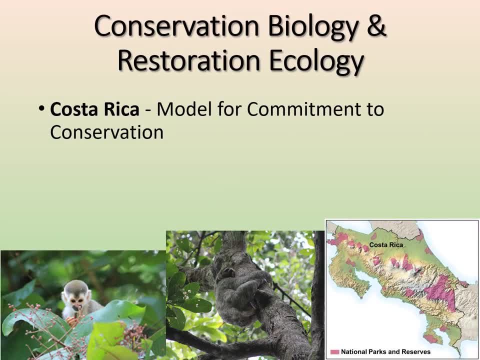 So, if we saw on that map, Central America definitely is a biological hotspot And so within Central America, Costa Rica- the country of Costa Rica- is really a great model for commitment to conservation. They put a lot of energy into conservation, biology and biodiversity, So they really encourage sustainable practices. 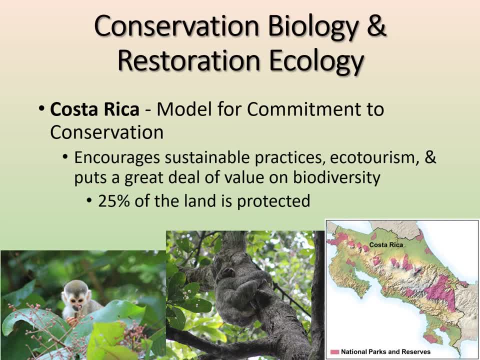 And so we have a lot of different areas in their country. ecotourism meaning bringing the tourism, bringing it out into the public eye, right And showing off like what you're doing and being able to have people come see the type of biodiversity in the area. 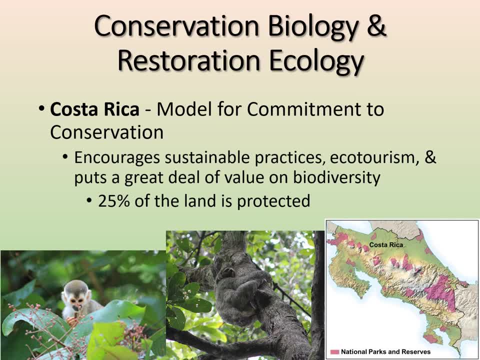 And they really put a great deal of value on biodiversity, So it means a lot to them And they really care about maintaining and supporting the biodiversity, sustaining their biodiversity. So 25% of Costa Rica is protected, which is great. So if you look at the map, 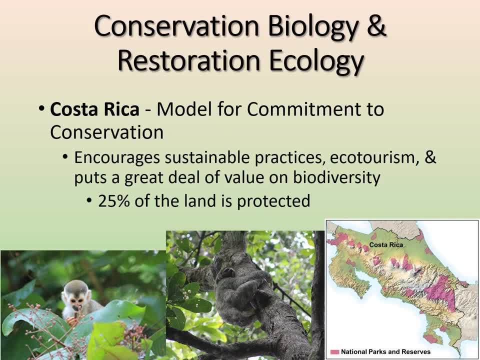 there's national parks and reserves all over the country And so they really are trying to do a lot of work in the conservation biology world And it's a beautiful place. If you've never been to Costa Rica, I highly recommend it. That kind of goes with that. 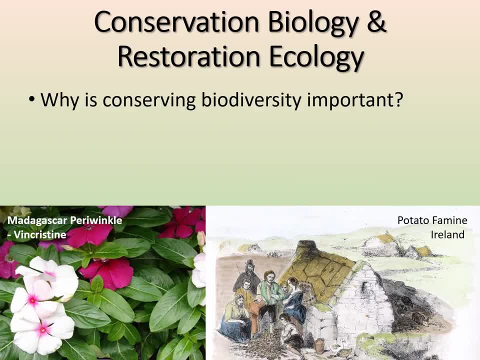 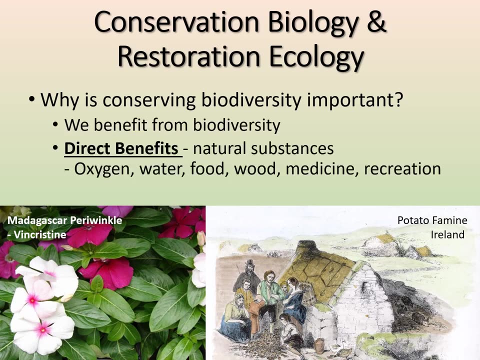 ecotourism idea right. So we've talked a bit about why we care about biodiversity and why biodiversity is important. but why is conserving biodiversity important? It's very similar, right. We benefit from biodiversity as a species, right? 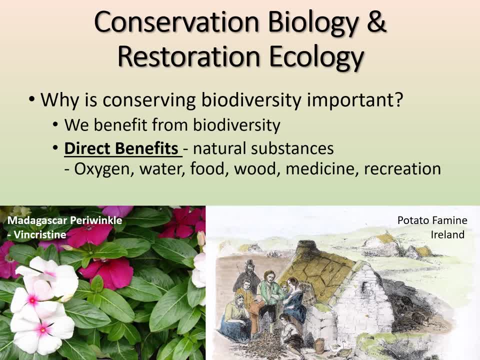 So it's kind of a selfish reason to care about biodiversity. Obviously you can. there are many selfless reasons- helping the animals and the environment and all of that- But ultimately that helps us as well, because we get direct benefits from biodiversity. 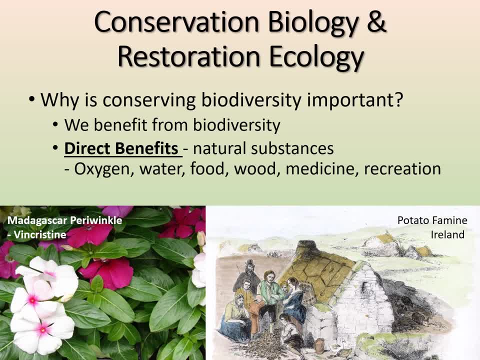 So we get natural substances right, Such as oxygen and water. Obviously we need clean water, We need oxygen to survive, We need food right. So animals- agriculture is all coming from, you know, animals and plants. We get wood. 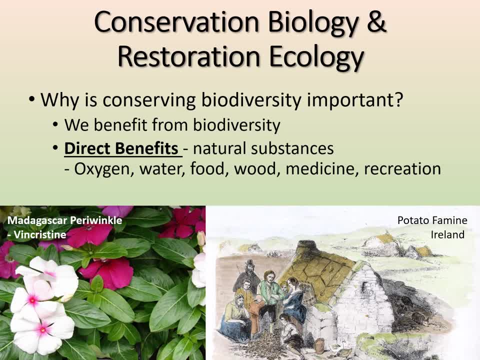 Right. So logging wood is very important in our world, but also things like medicine. So you may not think about it, but a lot of plants have medicinal purposes And so, just for an example, things you would never think about is this: Madagascar periwinkle. 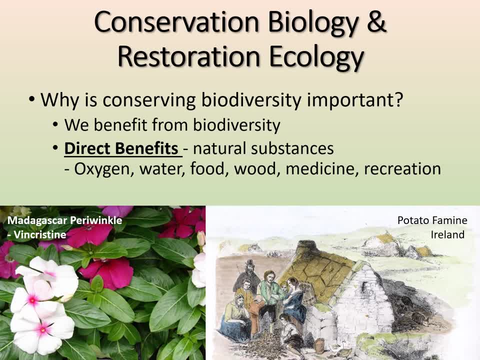 I have some in my backyard, They're quite pretty- Actually has a medical substance called vincristine, And vincristine is also a brand named Oncovin, which is a chemotherapy agent, So it's really the main treatment for leukemia. 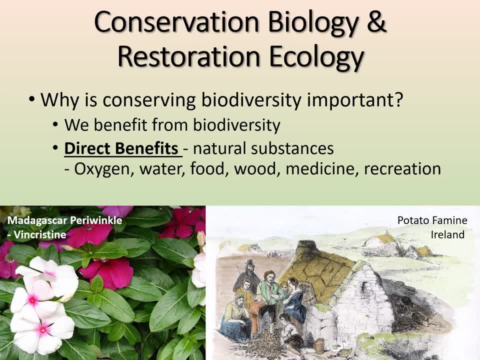 especially childhood leukemia, as well as Hodgkin's lymphoma, which is crazy to think about that. you know, one of the main chemicals for chemotherapy is coming from plants, right? So lots of medical reasons why we need biodiversity in plants. 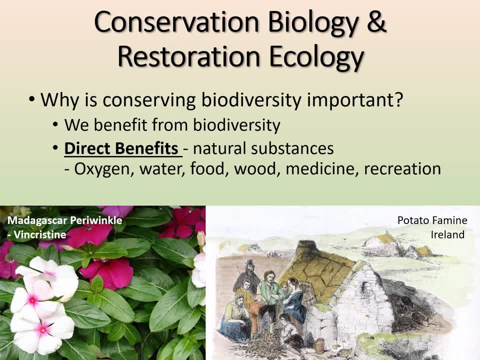 Another reason right Is the is recreation right, Keeping our nature preserves and wild and things like that that we can utilize right For our own enjoyment, But also going back to kind of agriculture and food If we don't have the biodiversity we talked about. 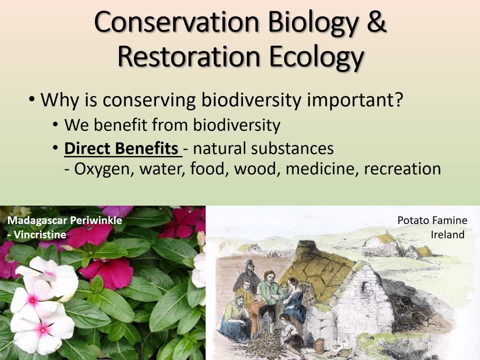 kind of genetics right, The genetic diversity earlier right In our last lecture And similar thing that's happening with the wheat over in in South America and things like that is the potato famine happened, So there was really only one type of potato in Ireland. 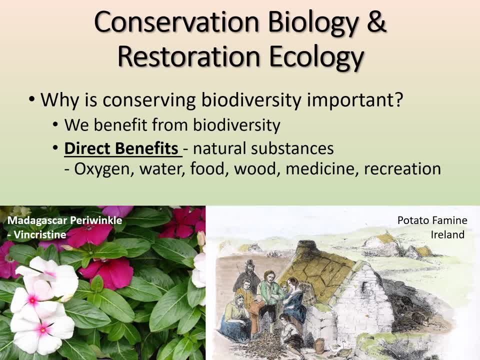 And they really, you know, sustained themselves on potatoes. And what happened with the potato famine is, when the potato, that type of potato, got a disease, it really wiped out all of the potatoes and then therefore wiped out a lot of people as well that were depending on those potatoes. 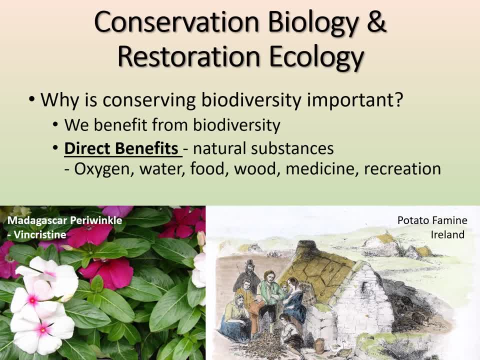 So if they had had a different type of potato biodiversity, maybe there would have been a potato that was resistant to the disease that the potato had in Ireland. So just kind of an idea there, where you know, agriculture and things like that are very important for biodiversity. 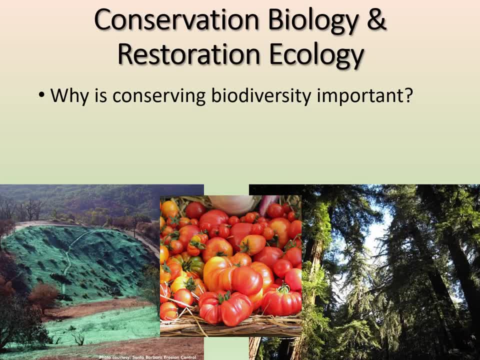 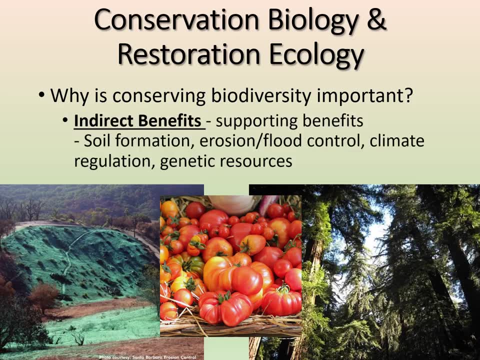 So not only do we get direct benefits like food and water and medicine and things like that, but we also get some indirect benefits as well. So these are going to be supporting benefits such as soil formation. So the soil is really going to help recycle nutrients. 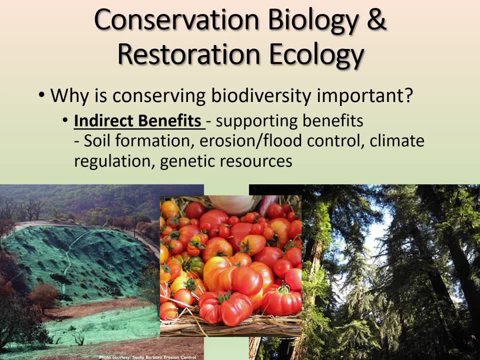 So there's microorganisms that are really important, but in the soil we have decomposers and those detritivores that break down the wastes and help with soil formation, and important soil, or good soil, is very important for plant health, Right. So plants, not only in the wild. 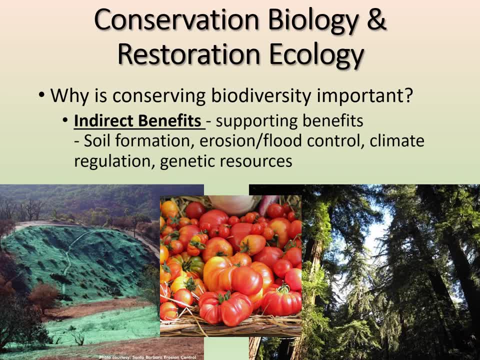 but also for agriculture too. So that's kind of indirect right. So it's not the plant itself but the soil that the plant is growing in. We also have erosion and flood control, So plants that are going to block wind, you know. 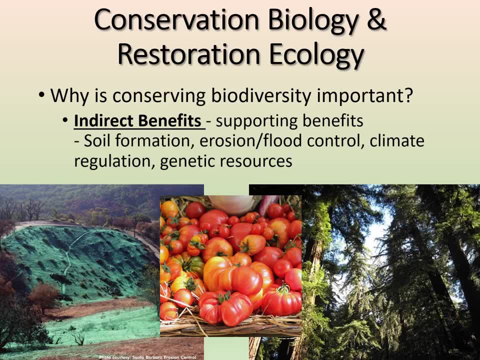 roots that are going to stabilize the soil and increase water uptake, things like that. So you know they try to hydro seed and hydro mulch after fires- right, That's that green stuff and sometimes maybe different colors that they blow onto the soil. 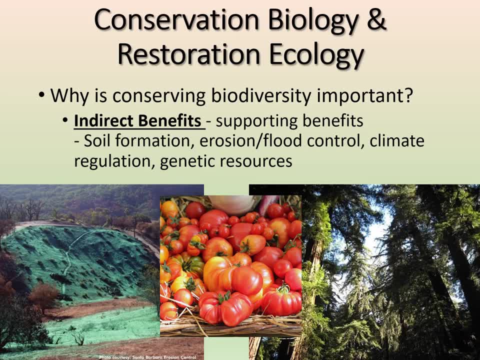 so that they, hope fully, can restore the plant life in the soil after a fire. Also, we have climate regulation right. So plants, communities of plants, provide shade, reduce the temperatures. They help wind breaks, things like that. They take up CO2.. 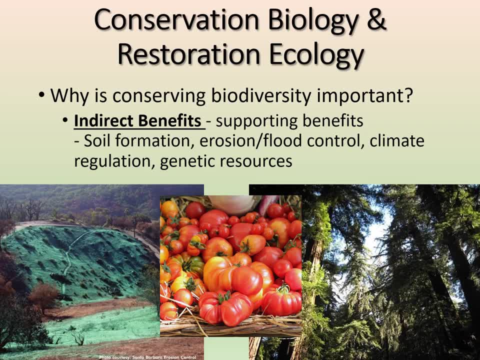 All that is very important for creating, you know, a good environment for not only other plants but also other animals as well. And then genetic resources, right, So genes that we can transfer or breed into to our crops that are going to help with nutrients. 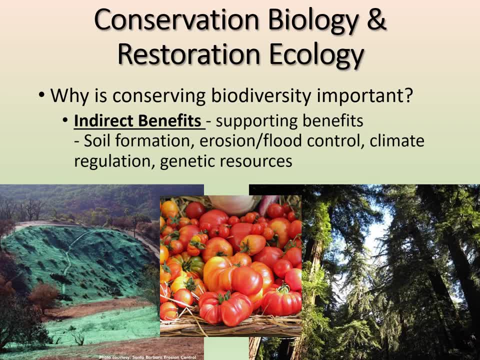 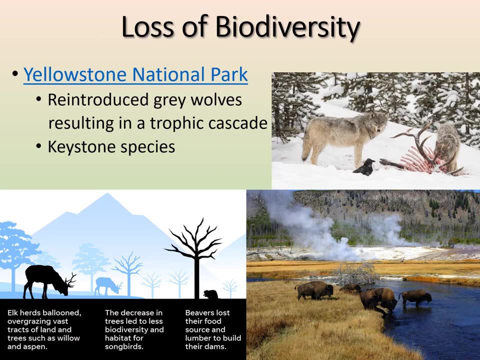 growth abilities, things like that. So kind of that genetic engineering we've talked about before. So these are all kind of indirect benefits that kind of go along with our direct benefits. Okay, So what happens when we do lose biodiversity? So we've talked about our threats to biodiversity. 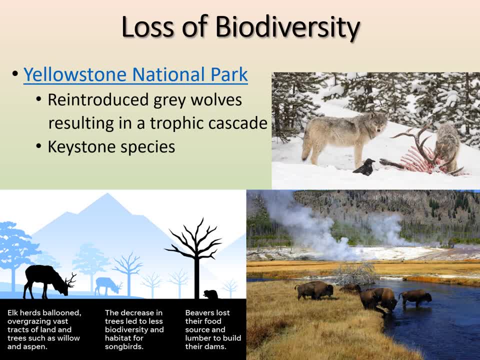 We've talked about conservation, biology- How do we combat those threats- But what actually happens when we lose that biodiversity? So hopefully you guys were able to do this assignment last week and research a little bit about the Yellowstone wolves in the National Park And what happened when those 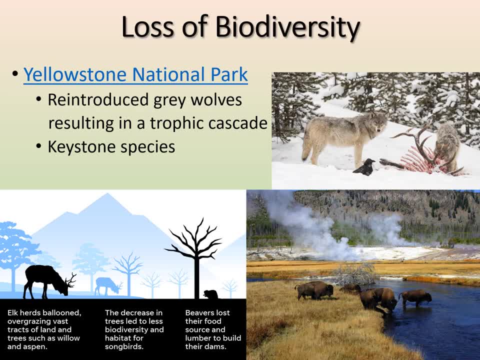 when those wolves were hunted, you know, not to almost to extinction, but very, very low numbers, to where we almost removed the wolves from the trophic feeding levels, right out of the ecosystem. And so what happened? are the elk population really increased? 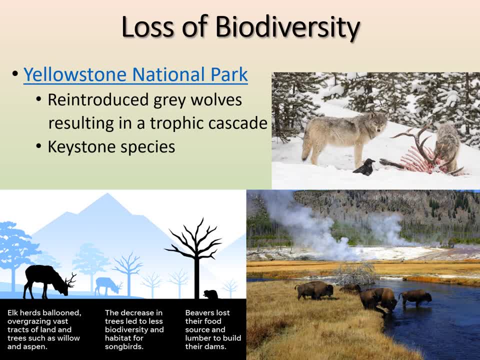 right. So the wolves usually hunted and ate the elk and kept their numbers in control. So the elk population just ballooned and really overgrazed a lot of the land and trees, such as the willow and Aspen, And so with this decrease in the trees, 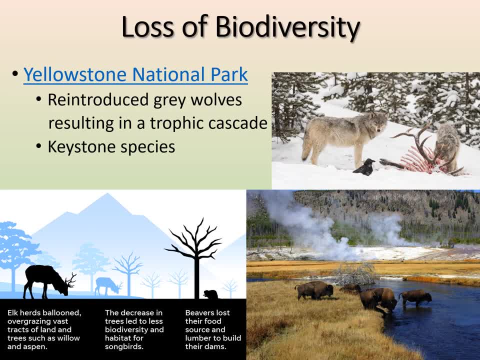 it led to a loss of biodiversity and a loss of habitat for a lot of songbirds, But it also lost a food source for beavers and resources to build their dams, And without the beaver dams, then you're affecting the water quality and the biodiversity within the water ecosystems as well. 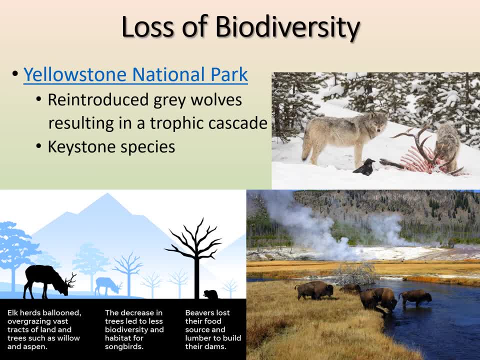 So it was this huge cascading result of a loss of biodiversity within Yellowstone National Park, And they realized this, And so then they reintroduced gray wolves to try to restore the trophic cascade and that natural balance of all the species in the ecosystem. 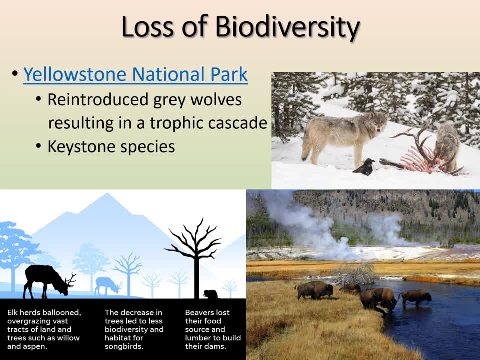 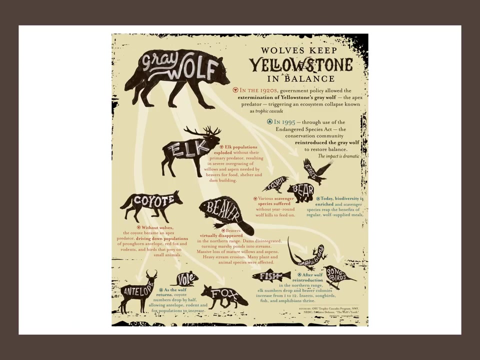 So we do consider the wolf a keystone species in this ecosystem because they increase biodiversity. So remember, keystone species are positive and they increase biodiversity and without them you get a loss of biodiversity. So here's just what happened, right that we just discussed- with the gray wolf in Yellowstone National Park. 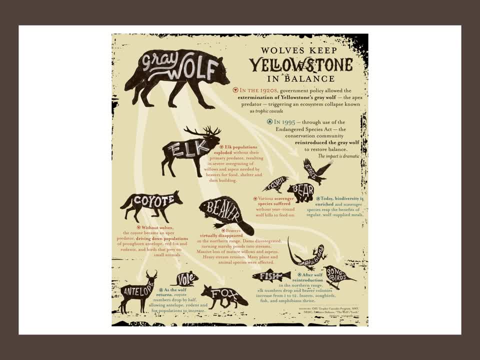 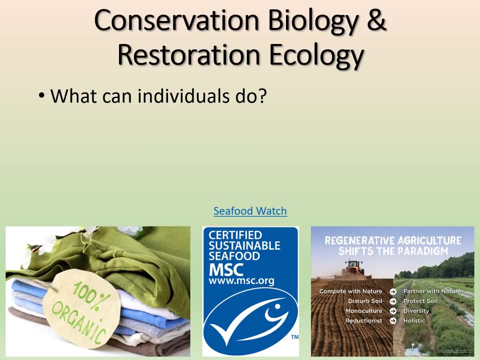 So you can read through that and how it affected the entire trophic cascade that we just discussed, And hopefully you guys were able to talk about this a little bit last week as well. So, after talking about all this conservation biology and threats to biodiversity and why it's so important to try to maintain and increase biodiversity, 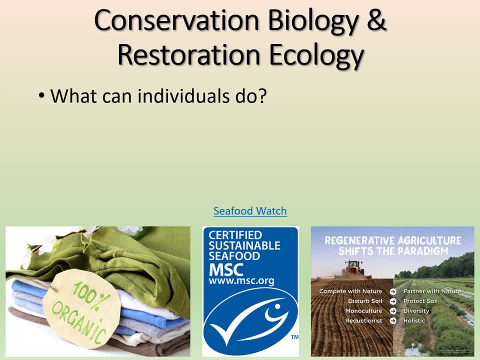 So that's all for today. Thanks for your attention. what can we do as individuals, right? obviously there's going to be a lot of organizations out there that are really dedicated to conservation biology, and if you're interested in it, then i definitely recommend, you know, doing a lot of research and seeing if there's any. 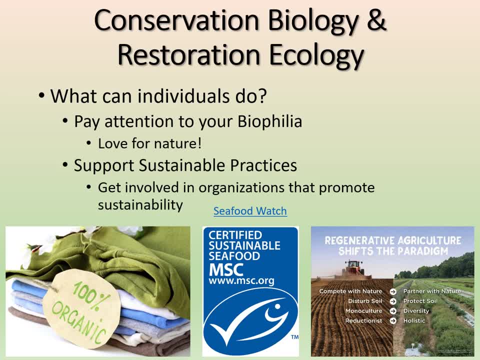 you know groups or anything that you can join, organizations that you can join to help restore biodiversity. but what can we do right, just in our everyday life? you can kind of just pay attention to your own biophilia. biophilia is just the love of nature, so just pay attention to. 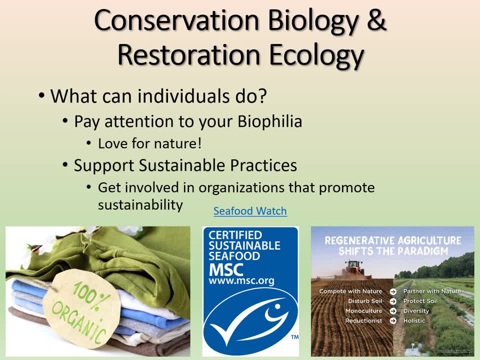 your own opinion and feelings on nature. you can support sustainable practices, right, so you can get involved or at least research organizations that promote sustainability and you can support those groups and organizations. so you know things like going organic, things like that. there's a whole seafood watch where you can actually um, you know, certified sustainable seafood. 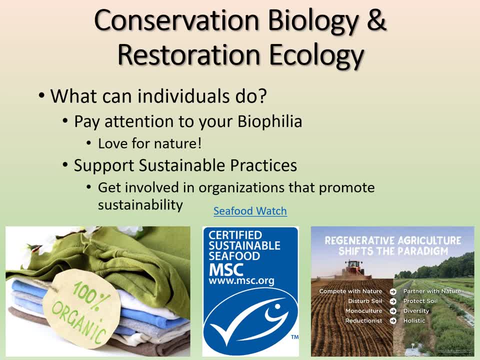 so how the seafood is caught and everything. that's a big one, because right now there's a huge loss of biodiversity in the oceans due to over fishing, that over harvesting problem that we discovered earlier. so if you know kind of what types of seafood to look out for, um, that can just be. 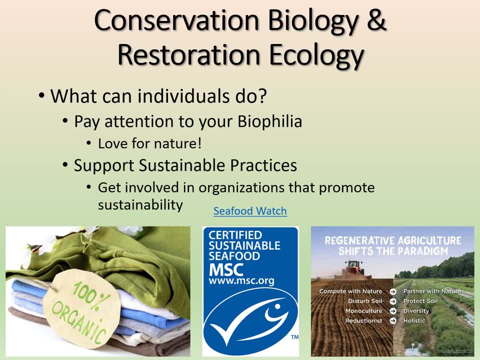 something that you do when you're, you know, just be more cognizant of it. um, a big thing that they're trying to do in agriculture is kind of shift from, uh you know, this competing with nature idea to more partnering with nature for agriculture. so you're trying to protect that soil formation and